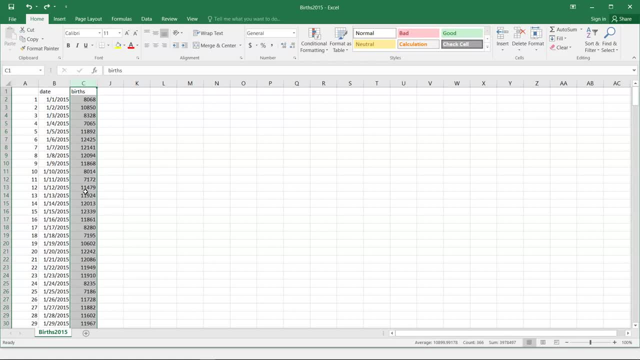 over a period of time And, uh, that is one of the important stream within the data science project: to know how you can calculate the time series for a casting. So, in a nutshell, the answer I wanted to give you is that, whenever the data is collected over a period of time, that is basically nothing. 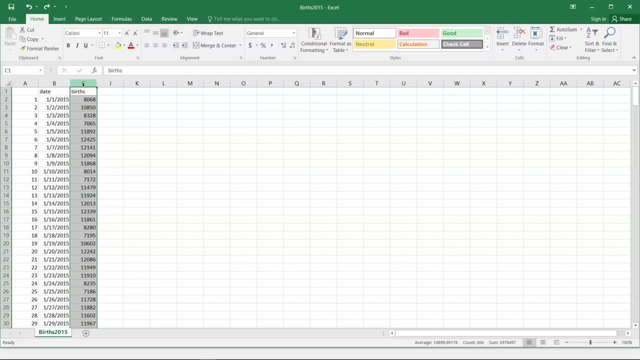 but the time series, And for that you need to use the time series modeling approach for the uh, for doing the data science project or for the forecasting of the future values. All right, So let's go back to the Python, the Jupyter notebook. So for that, what do we need is: 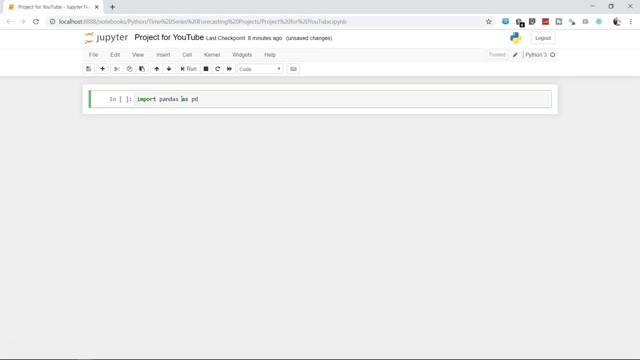 basically a couple of libraries imports pandas, as, uh, that is our basic library. I will show you the uh, the library requirement, as and when it is arriving, uh arising, so that, uh, you will know why we are using a particular library, but two important libraries. 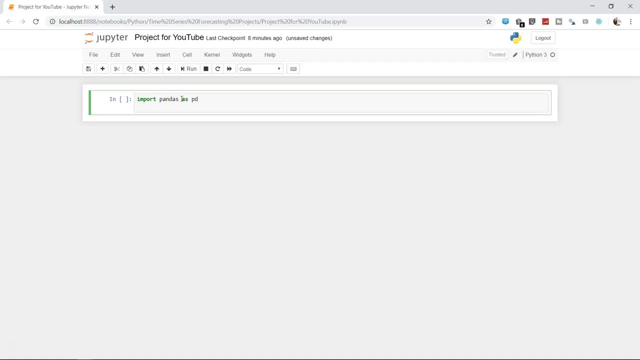 we always import is one is for data reading and one is for data visualization. So import, let's say the dot, uh, I plot as as PLT and magic common, which is percentage Matt blood leg, If you don't know. uh, this, this particular module, it's nothing but the data. 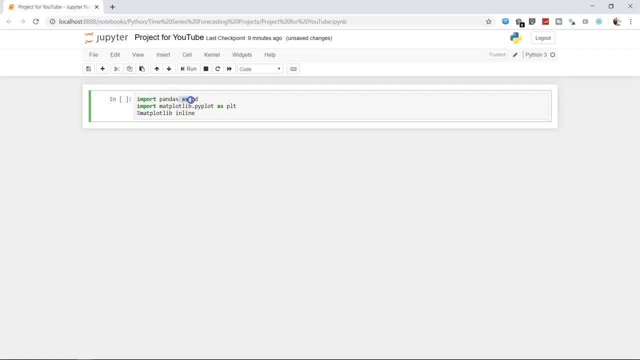 visualization module And what we are doing is using the as keyword, as we are specifying the alias. So this is just to keep in mind that you are completely big enough to use the as keyword, as we are specifying the alias. So this is just to keep in mind that you are completely big enough. 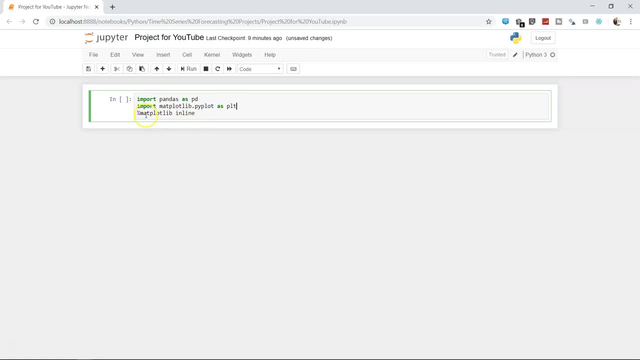 but if you already know, you can always skip this part. so after that, this magic command indicates that you want to visualize, or you want to display the plots just below the command you are executing, otherwise it doesn't display, or you need to use the command like plt dot show. so just to avoid. 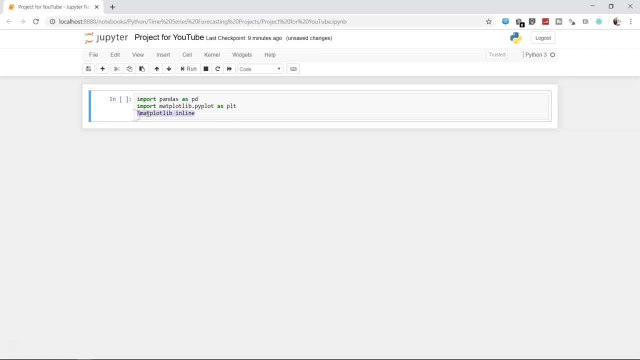 one command. we are having this magic, magic command which is %matplotlib inline, so let me execute this. and now it's just us warning that numpy and func size changed binary compatibility. i think we are good, it's just a warning we can ignore. after that, we need to first of all read the data and 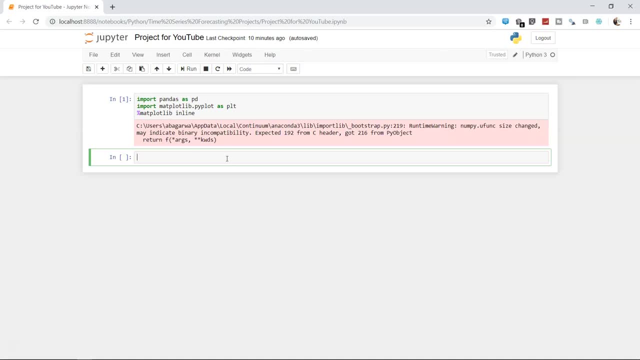 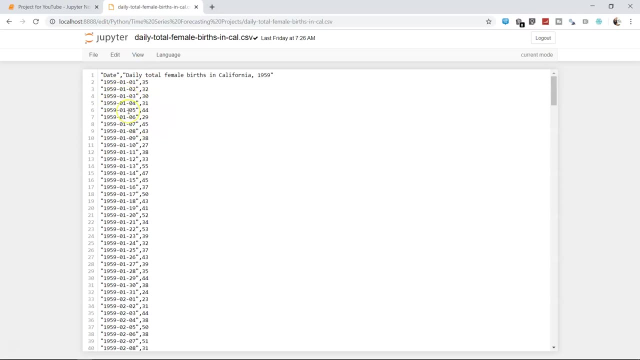 uh, what do i have is basically the same birth file which I just showed you, so let me just add one more column and paste the link. so this is what I have is basically the total, the date and daily total female birth in California, 1959. this is the. 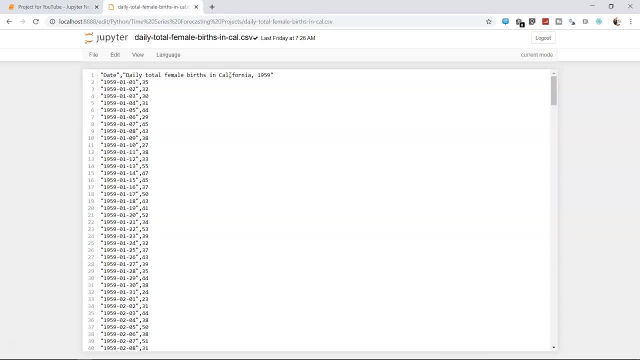 data that you can even find in the description. now, with this, I would, I would suggest that keep on viewing it, because we will continue seeing the, the, even the interview questions and the scenarios. you know, whenever you will see that, whenever I will figure it out that it is important from the 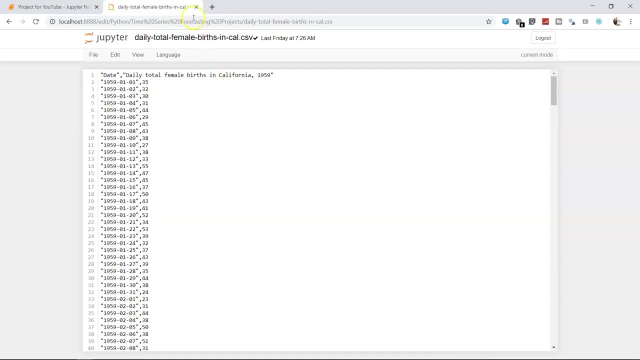 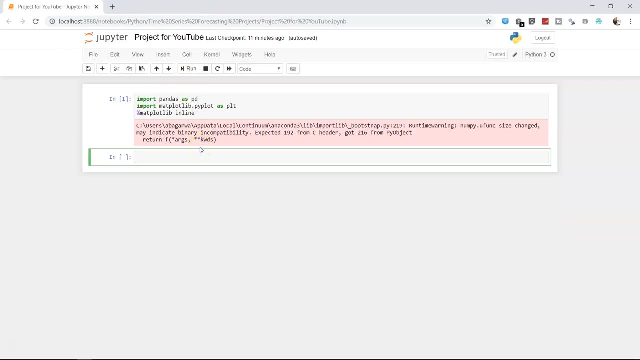 perspective of interview or from the project, crucial from the project point of view. so let me close this and let me read this data over here. so for that, what I will say is both or F underscore power, just to be very, very precise. this is object we are creating and PD dot read underscore CSV. 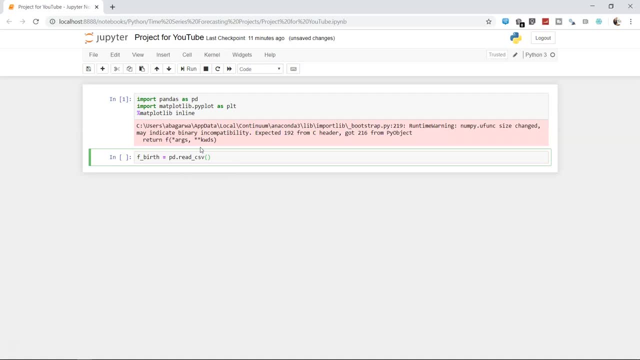 and in the CSV file, what we can do is read: first of all, specify the file name. so in my case, the file name is this: this is the minimum what you need to do. so let's see what happens if we execute this: no error, no warning, you're good. F underscore birth, and let's explore the data. so what I am going to write is basically: 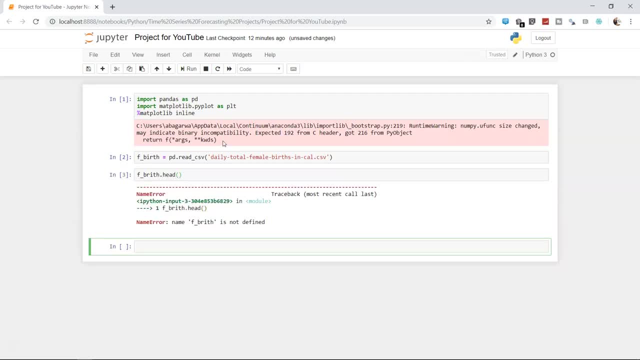 the head command which which shows the first five observations: F underscore. but be I, okay. and this column, date and daily total female number, that's the column, that which you, which you had just seen in another window which I opened it over there. so, and the first, this column, basically an index, 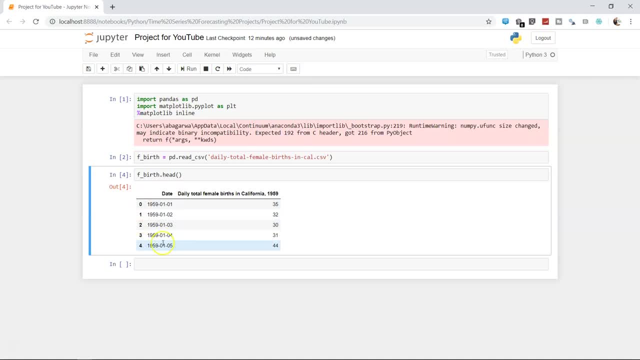 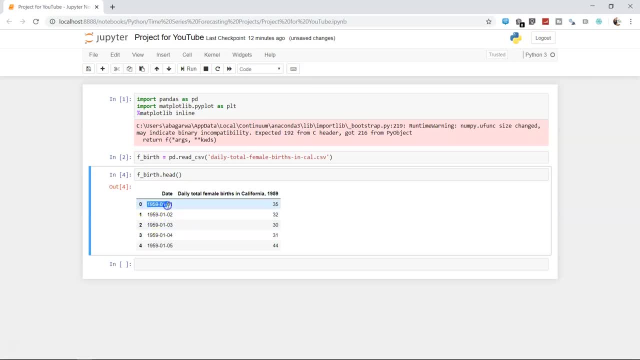 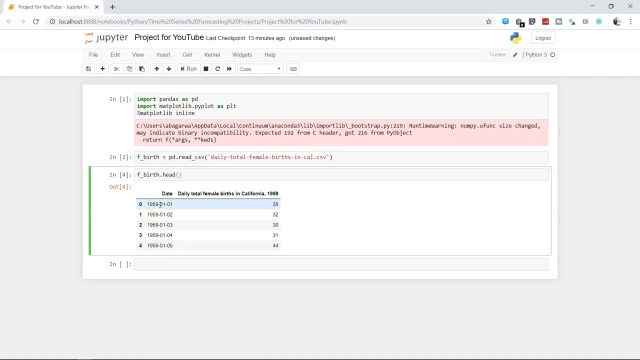 right now the date either can be performed over here of a means column and the next column can be executed over here. so some of you hot passed or not passed. but just to make sure that date is passed, that means Python or in this Jupyter Notebook when you perform date related operation or create an algorithm. 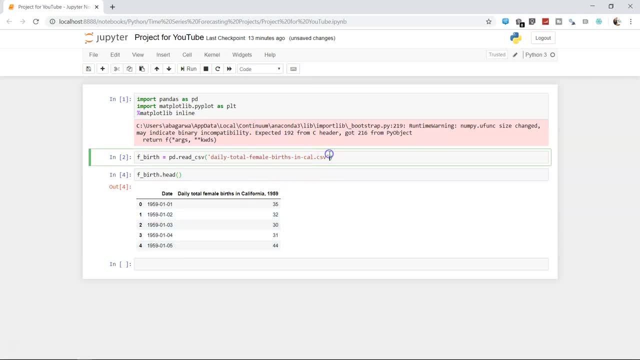 the date should be properly passed. So there are a couple of parameters that you can do. First of all, index underscore column. So index underscore call is nothing but specifying in which column you want to specify index. So just to view what are all the columns that are available, you can press shift and two. 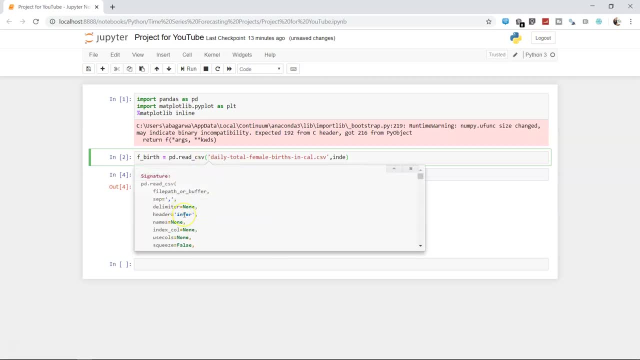 times tab, tab, tab and which basically shows all these different columns over here, And I just wanted to use the index underscore col, if I'm not wrong. I am not able to see the column, but there is this column which is index. 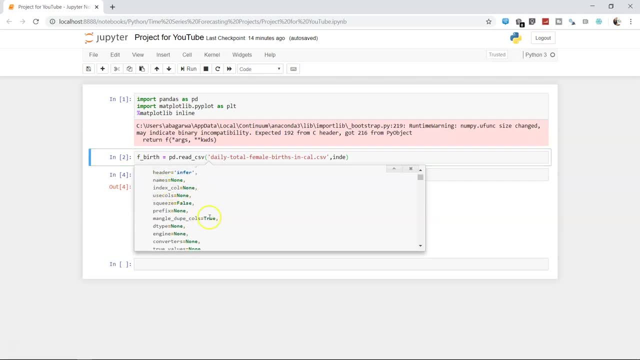 Yeah, there you go. Index, underscore column. Okay, So you can specify header. you can specify separator. by default it's a comma separated file, but if you have any other separator, you can specify this, and you can read this as well, because it has a lot of parameters. 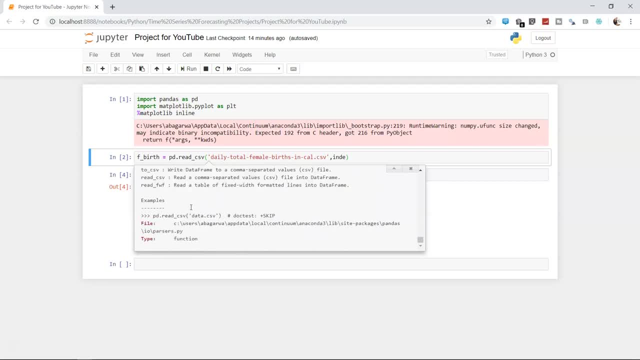 It has explanation for each parameter and I think down there it has some examples as well. looking at the file location. Okay, So index underscore call equals to zero. That means I want the first column as this Comma parse. underscore date equals to zero. 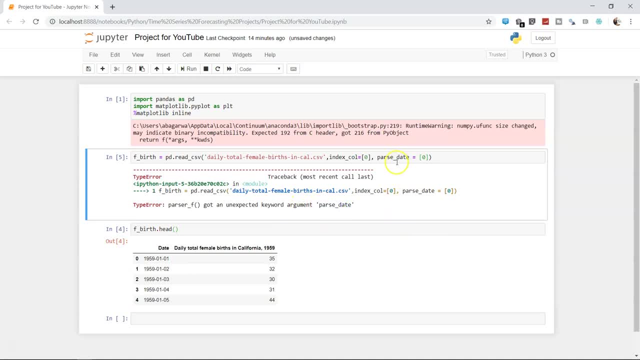 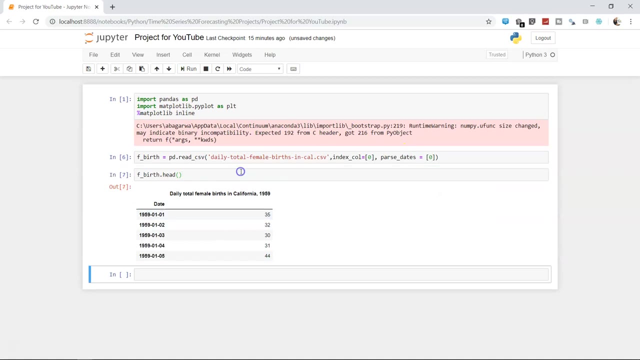 Let's see. I yeah, date underscore, parse or parse underscore date. Let me just quickly see what is the name of this. So parse underscore dates d-a-t-e-s. Now we are good. Okay, As you can see, we have date over here and female births California over here. 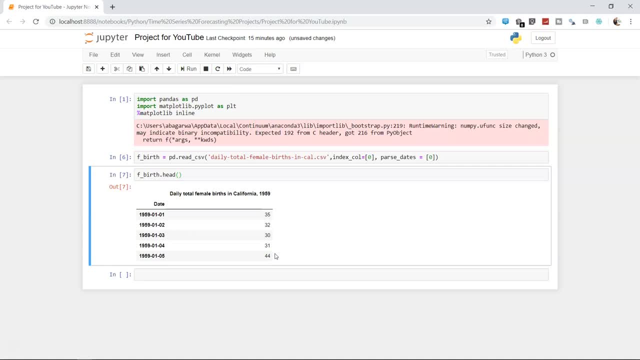 Now many times. you know there is a question which you will usually find- that if you have a data frame like this, then how you will convert into a series. This is a data frame, So there are two ways in which you can convert this into a series. 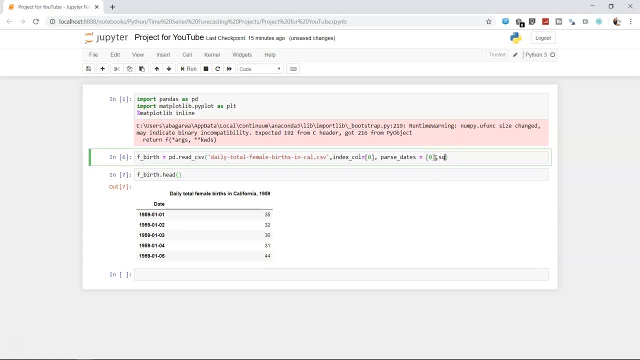 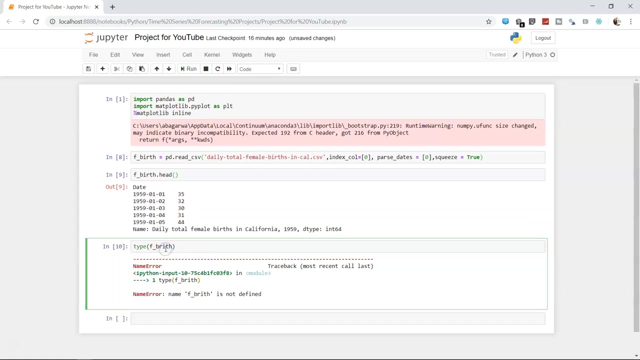 One is simply coming over here and saying squeeze- Okay. Squeeze equals to true. So now, if you see, this is converted into a different format altogether Right. Earlier there were proper column and everything, But now, if I look at the type of F underscore birth, why I am writing it wrong? d-i-r-t-h. 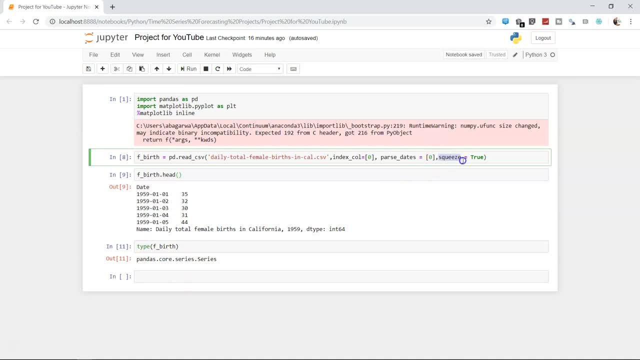 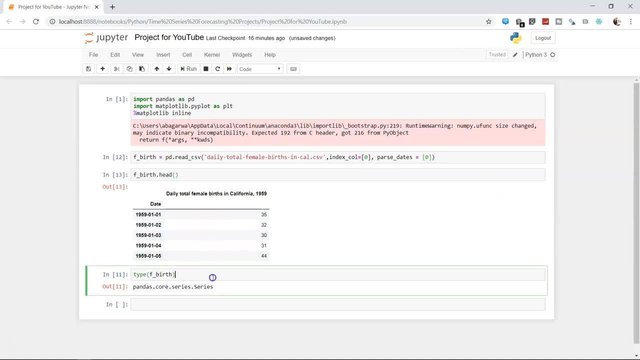 This is series, right, But if I don't have, squeeze equals to true. If you see, this is a different format which is a data frame Now. earlier it was series, but now, if I execute, it's a data frame. 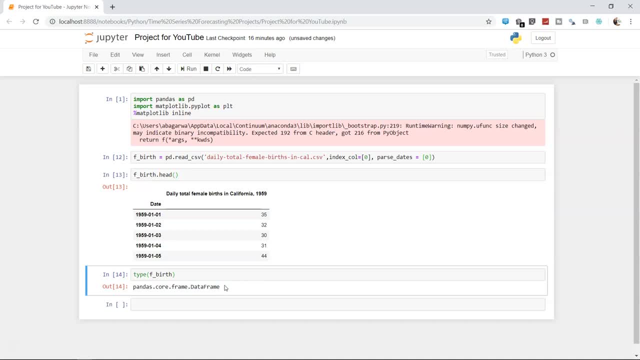 So data frame and data series is basically two different objects. Series is something you need for the time series analysis, But generally what happens is because there is a lot of data exploration and data manipulation, that is needed A data frame. Working on data frame is far more easier than working on series. 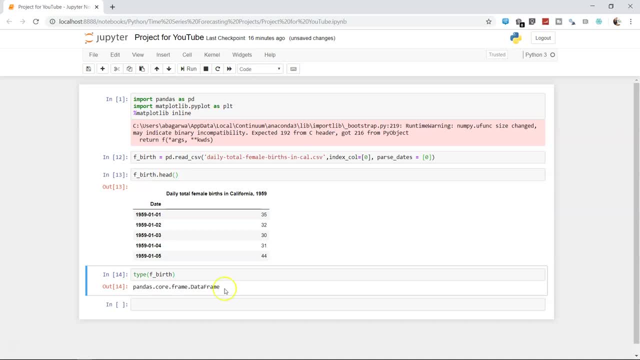 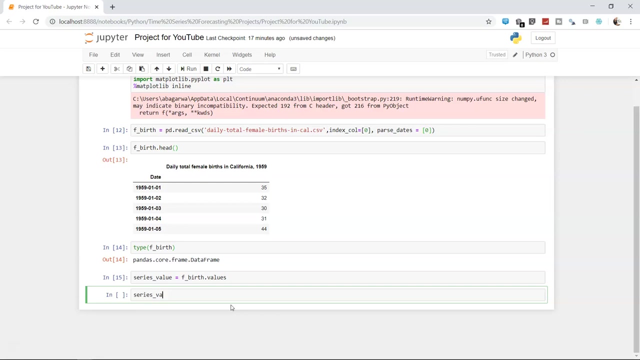 Once you are done with working with the data frame, you can always take the series out using the value method. So series underscore value equals to specify F underscore birth dot values. So once you execute this you can see over here Series underscore value. 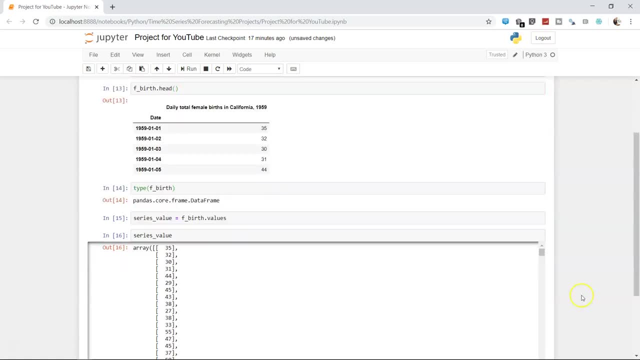 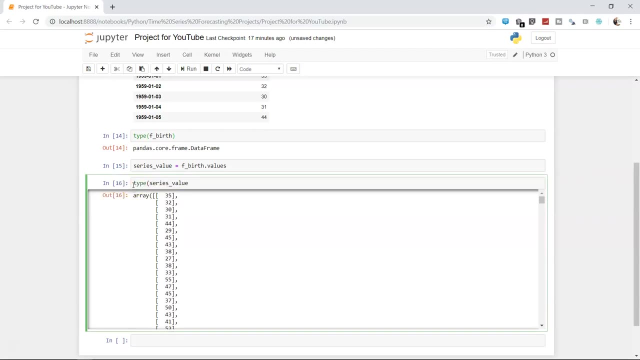 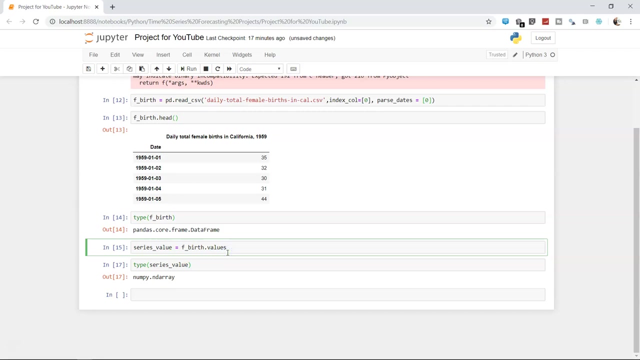 Okay, If I execute, it's basically an array which which the algorithm needs, And if I put a type over here, it is basically numpy nd array. So this, this values function basically helps us taking it out. upper series value which. 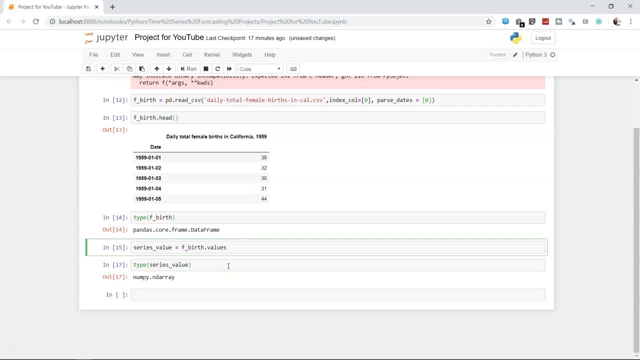 is this- into an numpy array which the algorithm usually picks up or needs to to do the forecasting. So Whenever the question comes like this, then you can always answer about the different types in which you can extract the series or create a series and then how you can convert. 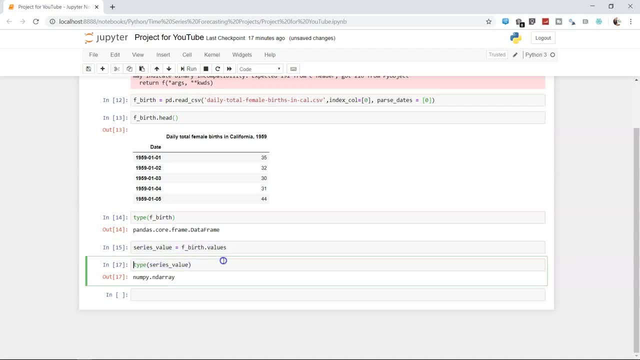 it into a data frame by using the values method. All right, So this is done, but what else we can do is basically, uh, the size method. I can show you just to indicate the size of the data frame. F underscore birth dot size. 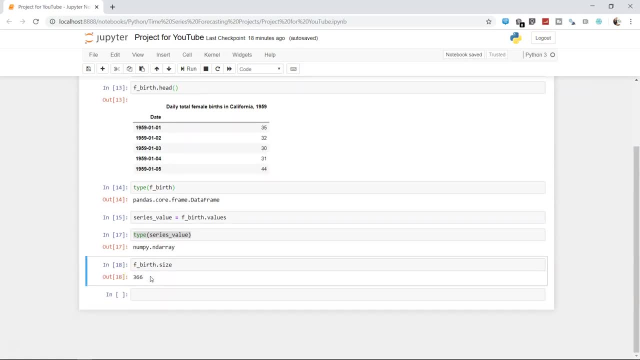 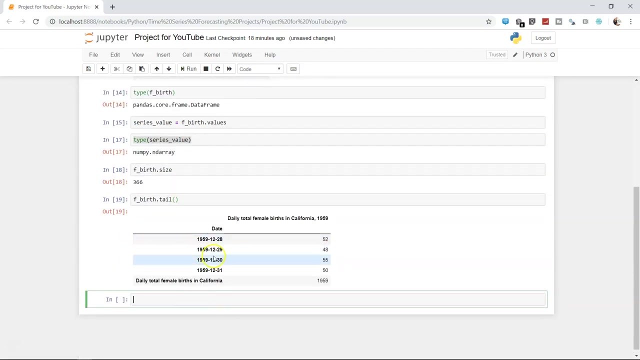 So what it indicates? Okay, It indicates that it has 366 observations And if we look at the couple of last observations, if you remember that had indicates the first few observations. but F underscore birth dot tail method is something where you will see the last couple of last information. 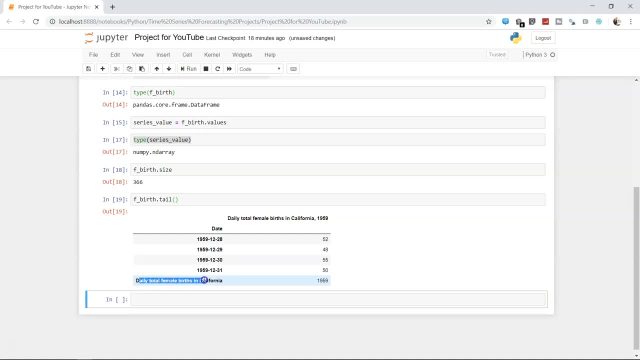 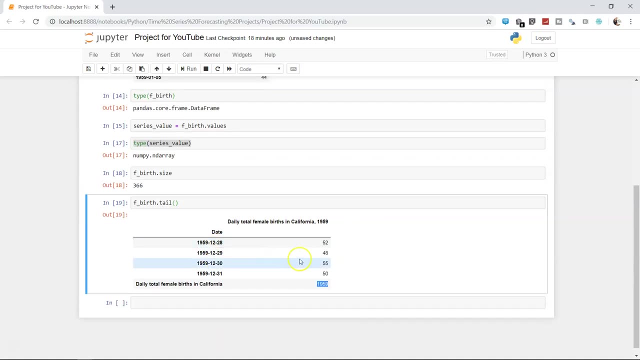 And one thing very interesting which is coming over here is the total female births in California 1959, clearly an outlier right, Because if you see for every date when some something, these are couple of last observation. So this is somewhere around 55,, 52,, 48.. 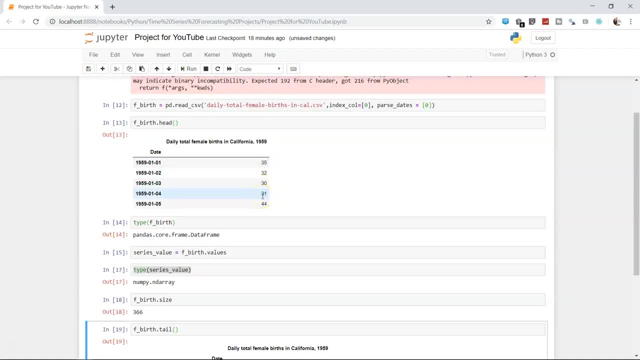 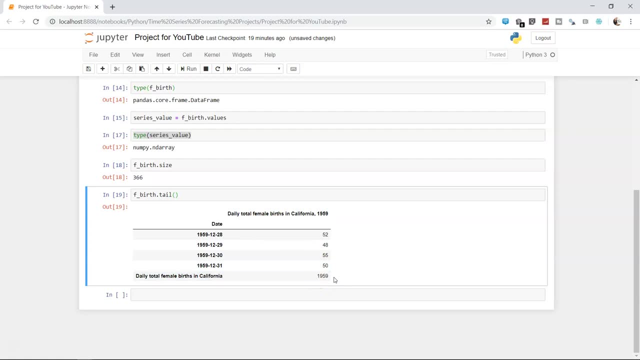 And similarly, for first few observations, it was around anywhere between 30, 30 to 44. So 1959 is clearly an outlier And that's why you really need to see the first few observation and last few observation, And not only this. you have the map. 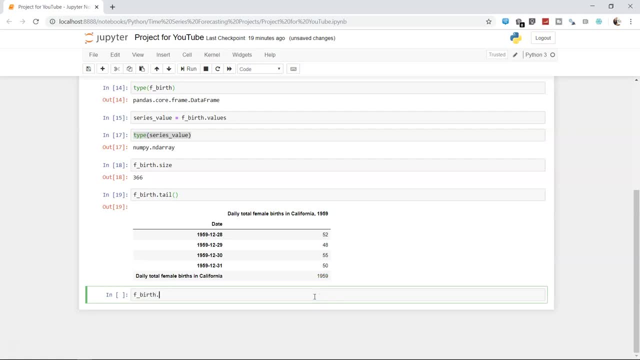 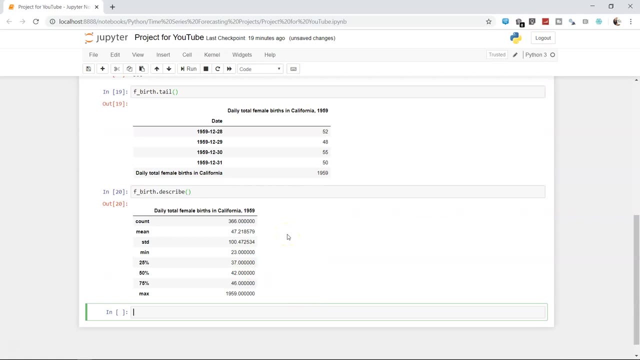 Which is F underscore: birth dot. describe So what it does. it described or creates the statistic for the entire data set, which are very crucial. For example, count: that means you have 366. count: What is the mean? 47?. What is the standard deviation hundred, which is very high? 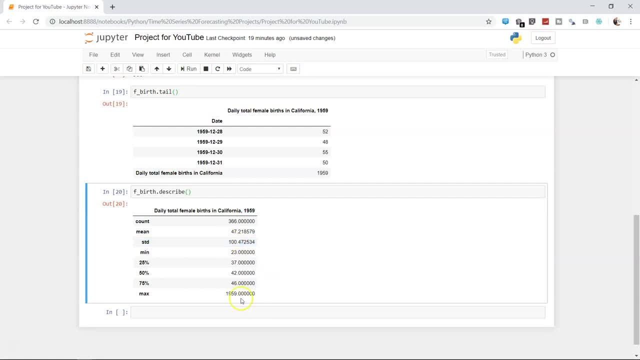 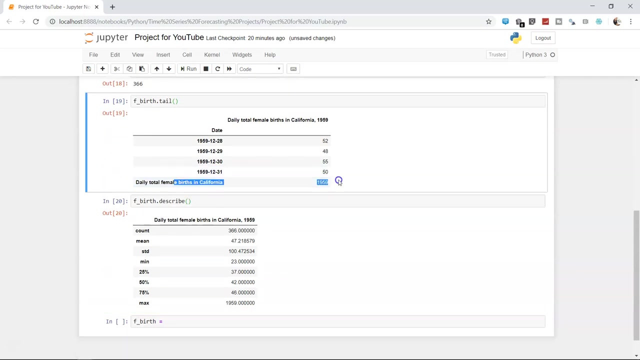 If you look at the age perspective, and that is mainly because the maximum value is 1950. And that is definitely not correct. So to correct that, what we can do is we can write this command: where we select, where we do not select, the last row over here, where it is: yeah, over here. 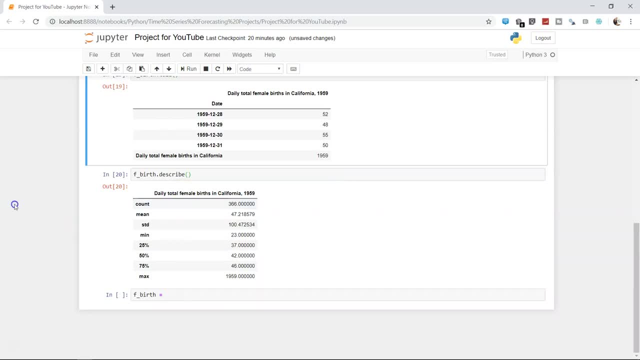 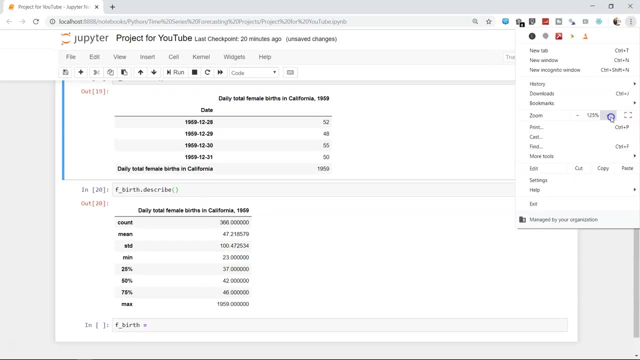 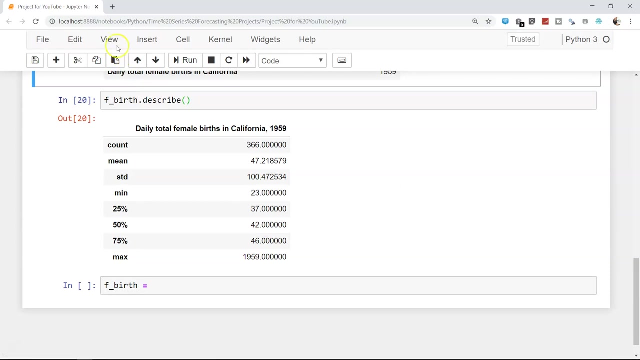 All right, And let me just increase the size in case you are finding it a little difficult to view it. Go here Zoom. Okay, Yeah, I forgot to do it earlier and I will just hide the header and I will hide the toolbar. 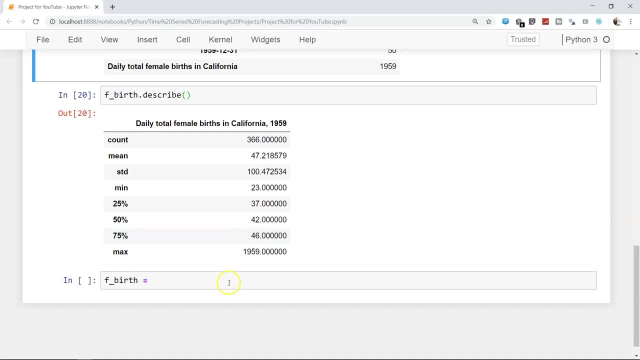 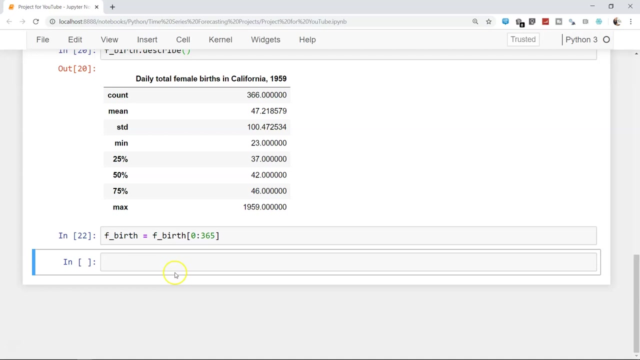 as well. Okay, Now it will be much more clear to you. So: F underscore birth, again F underscore, but right from zero to three: 65 F underscore birth, All right. So now, if I see Again, I'm writing it wrong. 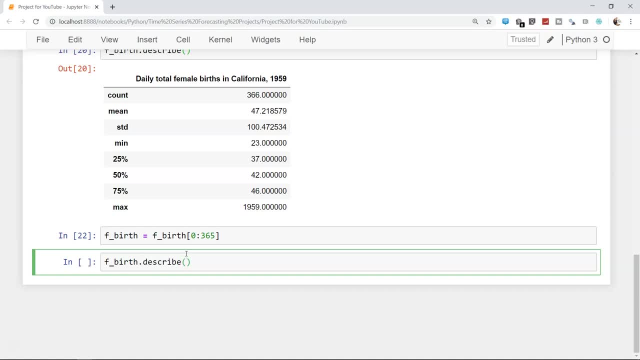 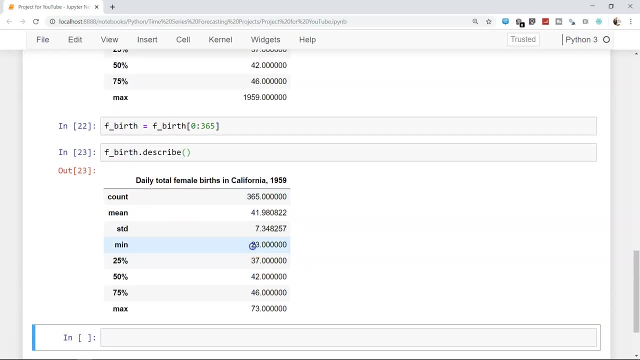 I don't know why just that doesn't go. that describe now, if you see it's very meaningful. So the minimum value is 23.. Uh, so minimum birth on a given day is 23. maximum birth on a given female birth is 73.. 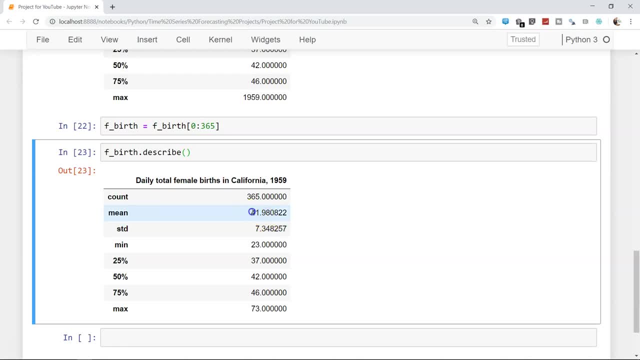 And the standard deviation. one standard deviation is seven and mean is 41 on an average, you know 41. But the standard deviation is three. So now let's look at the next one. Now the federal flexibility is 30. So let's say the company is planning a five month period where you want to have a child. 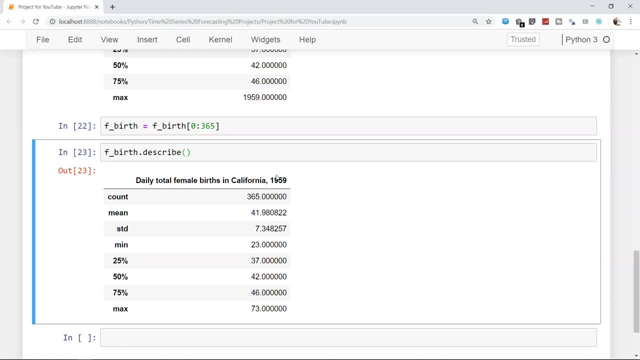 and you want to have a child for the rest of the year. So you've got a child to be born. You can have a child for three years. You can have a child for three years at a time. Now, if you're in aウи, you know for any say for a year and you're in a a year and 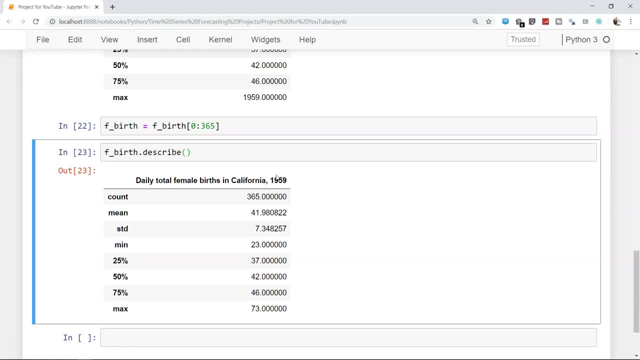 you have a child. with aываем you can have a child for three years or even length of a year, And then at the end of the year you can have a child. So at that time they're going to have a kid and a fourth or five year old. 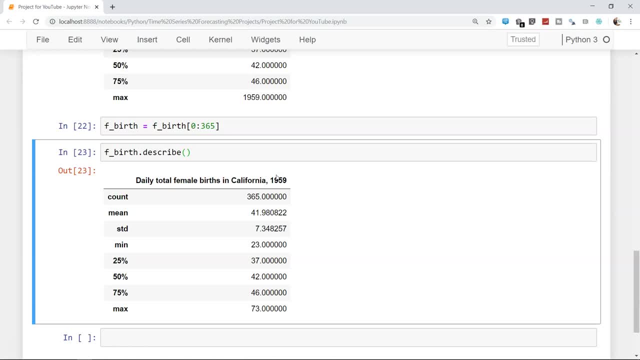 without even for a casting. with this information, you can even, you know, figure out what strategy your company want, if, if you are, let's say, in a market where you want to see how much new production of, let's say, dolls or barbie doll you need to do, or something which is related to the 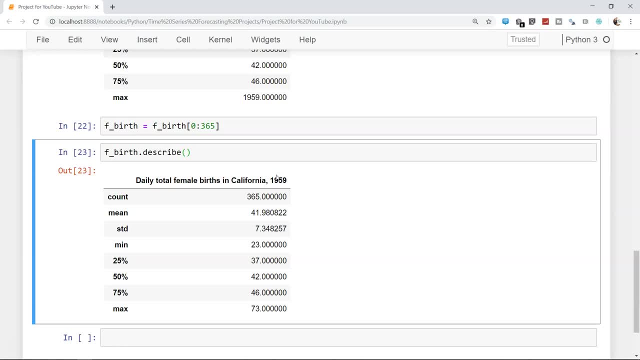 girls accessories because those girls, with as, as and when they grow, you know their needs arises and they basically go out in a shop and do the purchasing. so with this you can clearly understand how you need to plan your business. these are very economic factors that every company consider like. 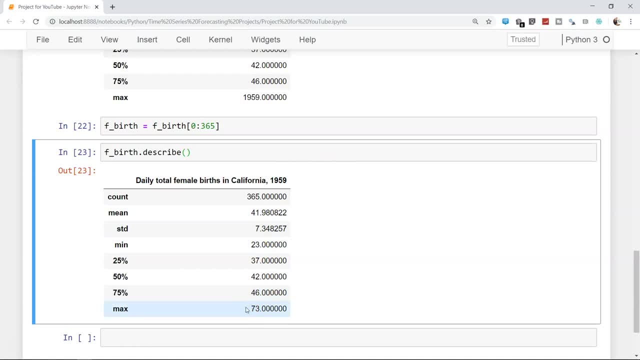 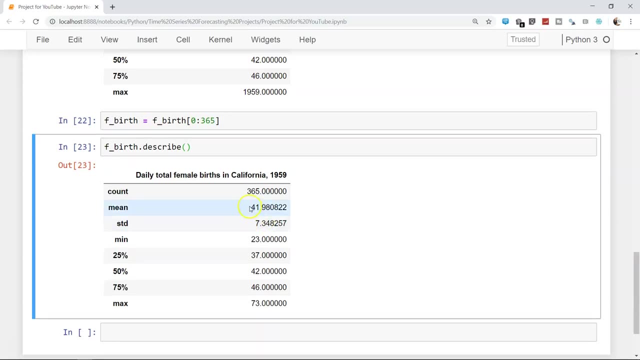 the minimum maximum standard deviation. all of this, and the most important is basically the average and standard deviation, because they reflect a lot that: what is the average value and how much it can vary it. or you know that there will be a variability in the value of the product. so the next part, after we have done this, is just visualizing the data. so 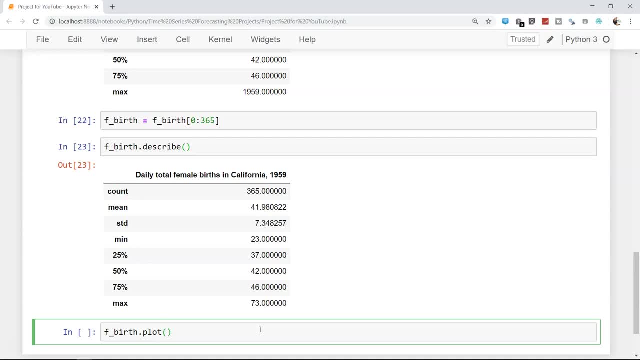 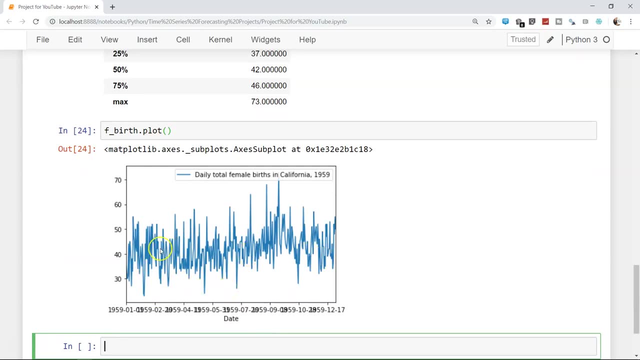 visualizing the data is very f underscore, birth dot plot and because we have plot in line already specified earlier, here is a quick plot. so this plot basically indicates that, yes, there is a variation in data there. you can see the peak, you can see the low point. so this, this indicates that 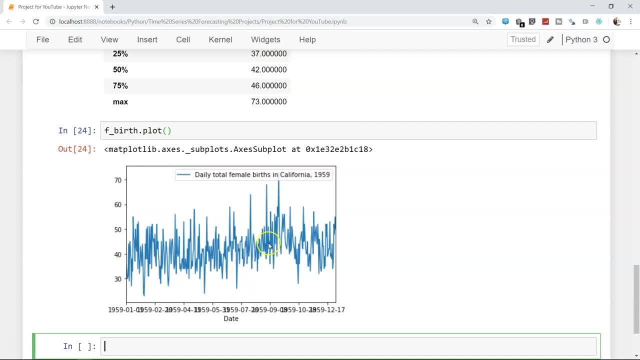 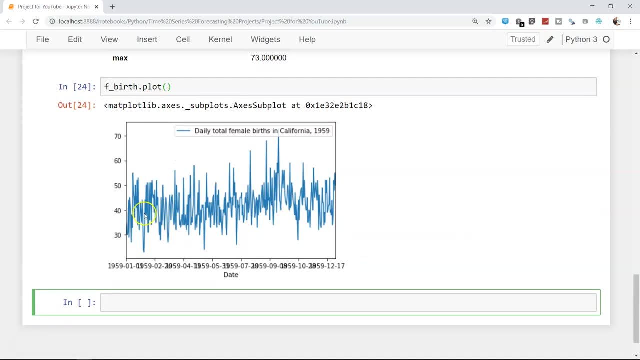 there is a variation of a trend over here, but not a very specific trend. uh, looks to me a bit of a stationary series. so this, this basically stationary, is something you will. you have heard it, or you must have heard it, when you have looked at the data science project and what it indicates is the series which 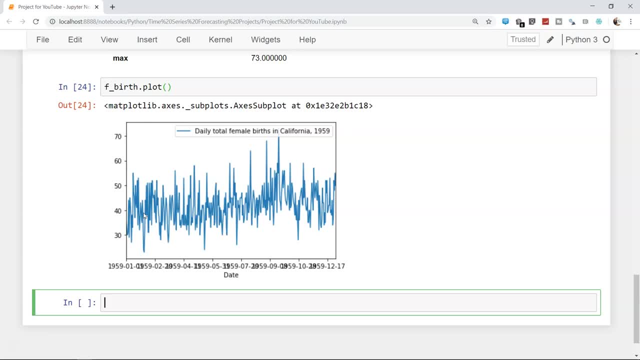 does not have any- uh, you know- trend factor in it and it is like a constant series with the constant mean end standard deviation. so this, this is important. the stationary series is important when you are working with the time series problem and the way we do that is to figure it out. the basically the 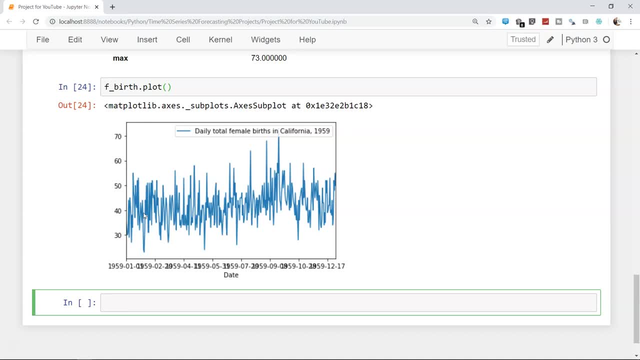 difference between the current term and the previous term, which we call it d, and i will show you in the in couple of minutes, that. what does this difference? order of difference, or the, the particular value d which i just mentioned? but before that, uh, the way we can much more clearer, clearer see this, these, uh. 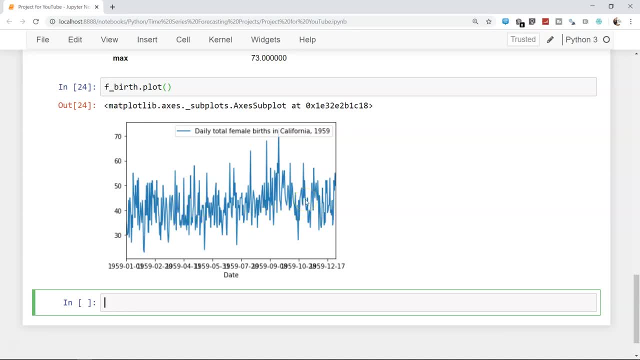 trend or this. this series is by smoothing the series. smoothing is one of the factors which you will hear, or you must have heard, when working or here you know, reading, about the time series uh project, so that the smoothing is basically taking up the, these values, and smoothing out with 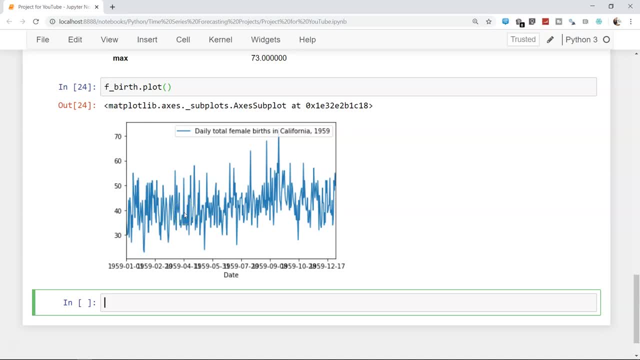 the help of moving air flow fridges. so moving average is nothing but uh, the moving average is taking a specific value in count. so, for example, if you are looking for a five day moving average, so you will start from the sixth day and the first five value will be the the. you will start from the fifth day and first five value will 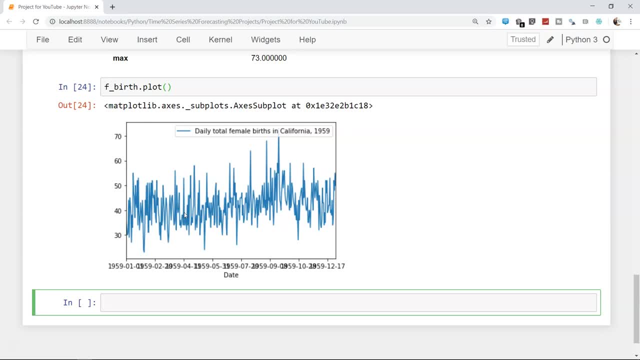 be the moving the average. the average of first five value will be the moving average for the first data point. and how you can calculate over here, here is: eh, theYA Leaderboard is f%h. mean for average is f, D i birth mean f to ga. 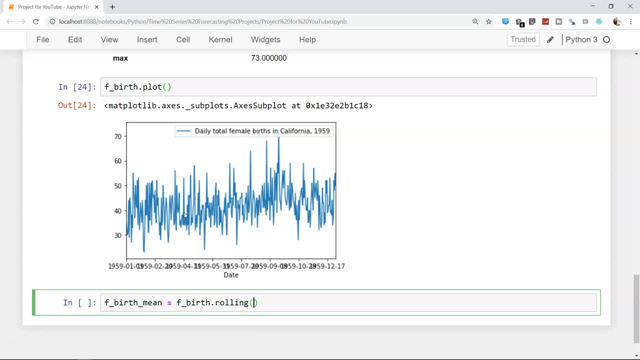 berj store, berdth dot wirtc. rolling rowling is nothing but the rowling five, day rowling 60, rowling 70, rowling 70, amount 1.. where, what, what? what was in that number 10 when rowling was 5, even to 16, early 17 days mean. 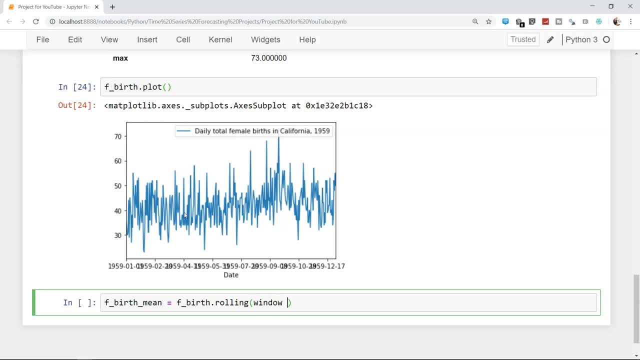 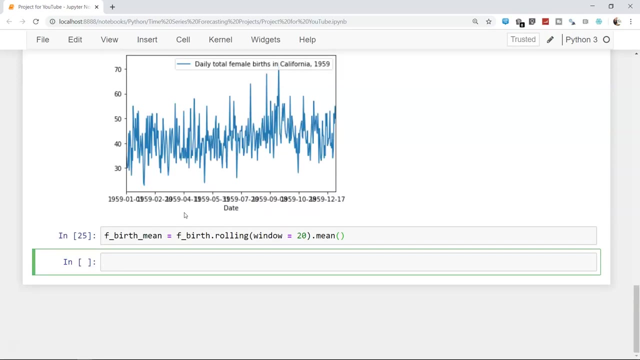 moving average value we want. so in that we need to specify the window parameter. so we can have 5, we can have 10, 15, 20- I have just taken the 20 and I'm taking the mean of it, all right. so this is how the value will be captured over here. 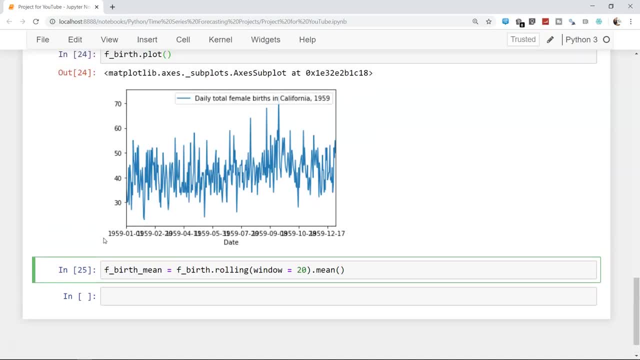 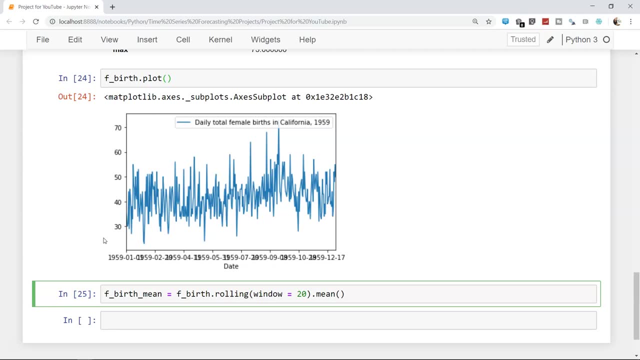 rolling fire 20 day mean for a 365 day period. I think that is quite doable because we have 365 data point and we are just removing the first 19 data points. so F underscore, birth dot plot. let me put it again over here: F. 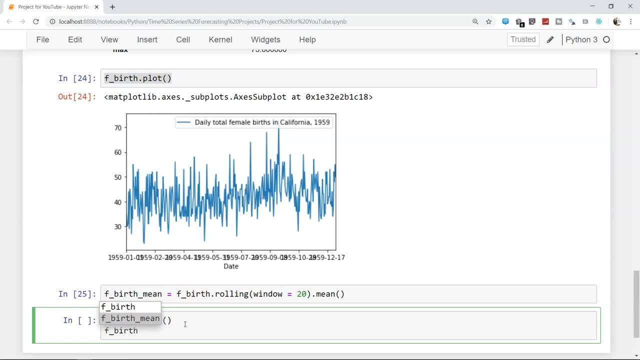 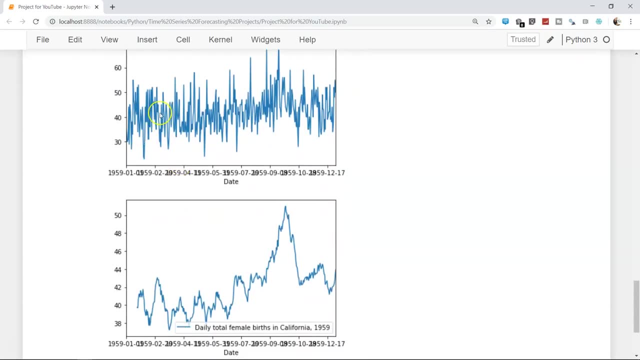 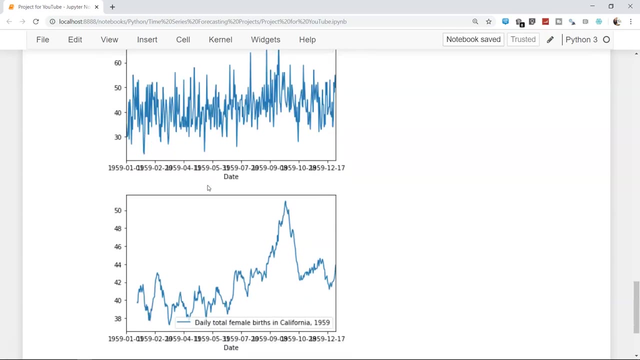 underscore birth dot plot. F underscore birth mean dot plot. and if you plot it, you will see this is the value which you have got as part of the actual series and this is the how your moving average is. so it's clearly indicating that there is a spike. 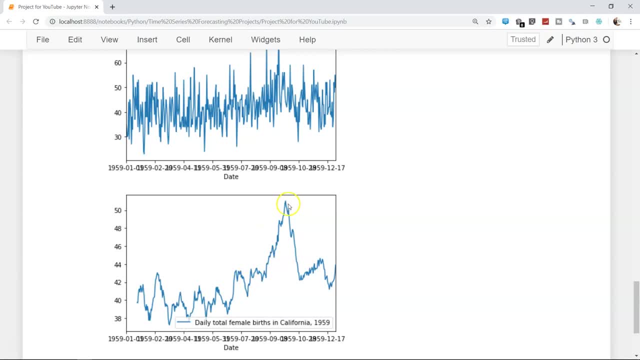 over here, somewhere around here, which is the later part of the year, and then it has come down and a very small trend. if you see little high trend which is clearly visible, which was not at all visible from here, that means the main series. so this way you can create the rolling 20 day average mean and 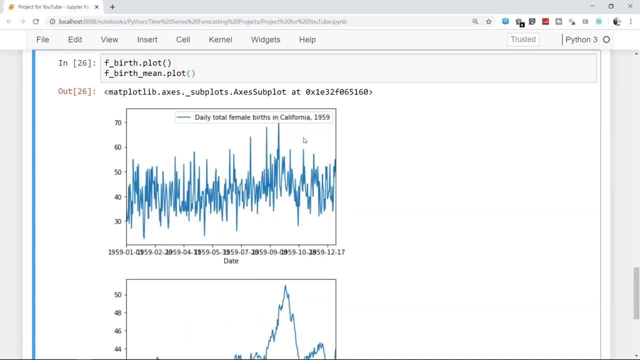 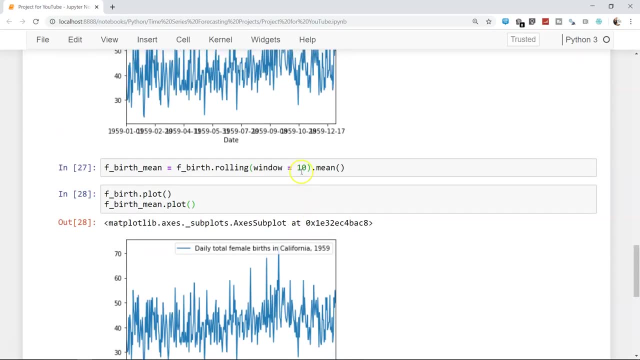 if I want, I can have like 10 days just for the experiment perspective and you will see. this is how the 10 day average mean. or if somebody is interested in 30 day, you can just change the value of 30 day, experiment with it and you can see. 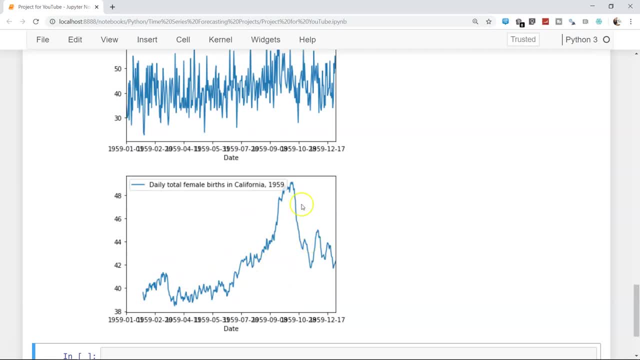 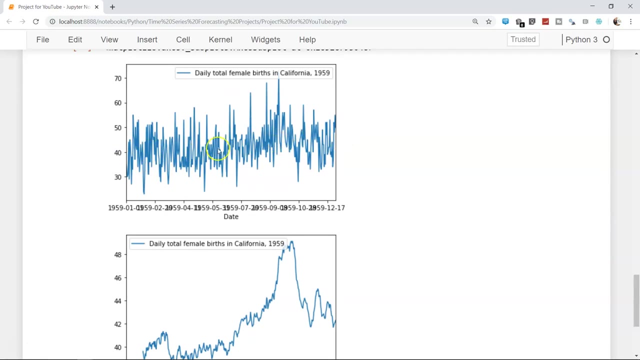 this is how the 30 day. as you can see, there is a lot of variation, but one thing which is clearly visible is bit of a trend and the spike over here. so very useful and helpful feature, just you know, to see the how you can remove all of this noise and see the clear graph and 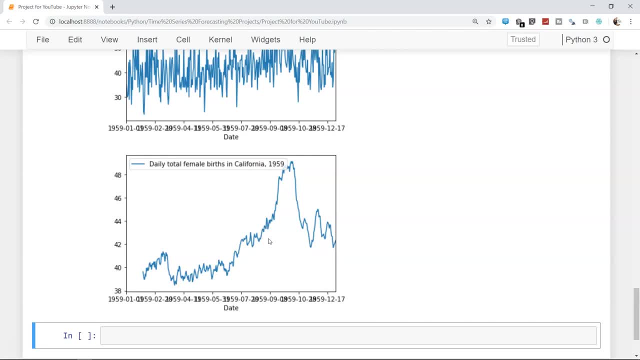 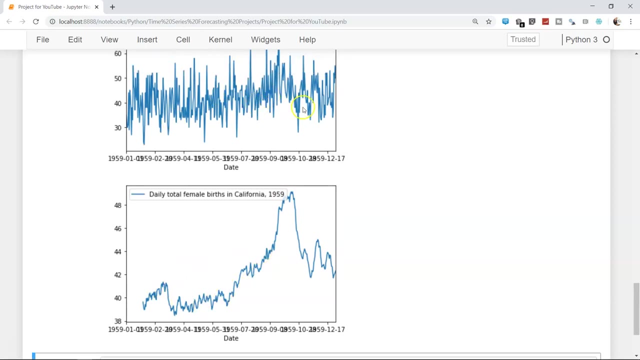 this technique a lot of time. this technique is used within the stock market analysis. if you have seen the chart of any stock, this is how they look like and the stock analyst used lot of moving averages to basically remove all of the noise, because there is a lot of fluctuation every day in the stock. 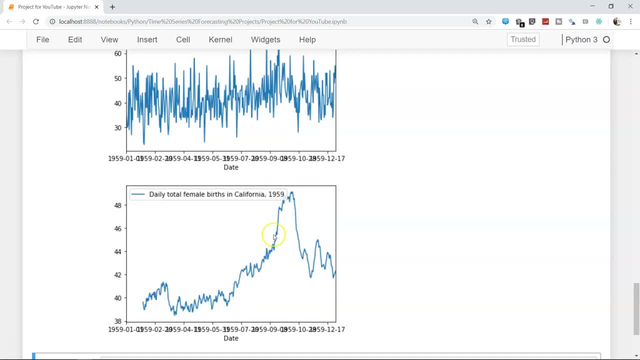 prices so they remove the fluctuation with the help of the moving average and for removing the shift. debeTube is also some chattel block in the stock market analysis. in the stock market analysis, the saver share share at the time series analysis. there are many other techniques and also affordable understanding and 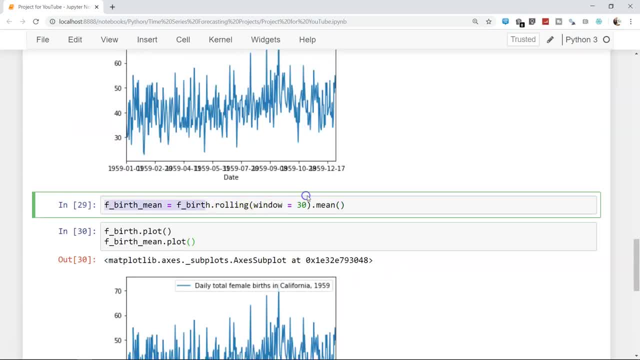 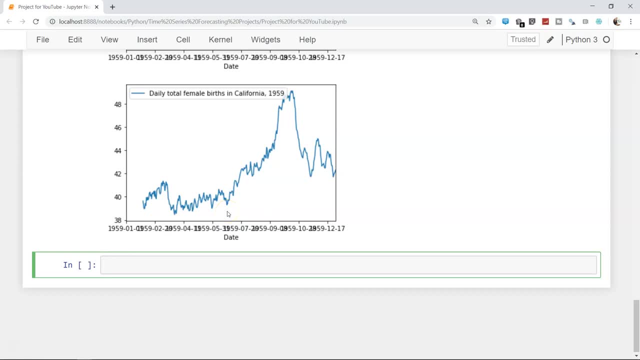 things to watch out for. but before we any steps, please don't forget- if you are interested in this type of Assessable Machine Learning videos also, there is a lot of place for우 course being hit by moving out inches. so this is how you can. you can basically do the moving average piece, and very useful because this- this even gets in a question about how you. 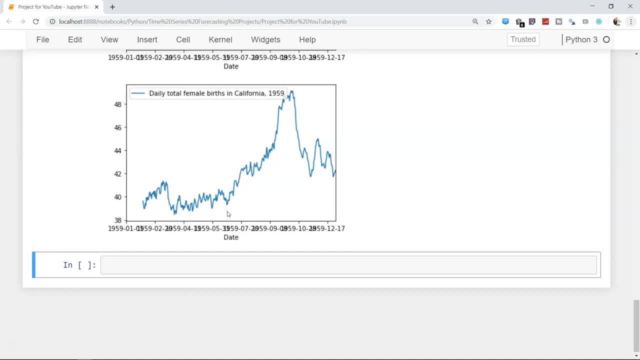 what is? what are those like normalization of the value, log transformation. there are other types of transformation that you can do on a project, but for this project i want to keep it very simple and for that i will just straight ahead, move to building a model so that you are 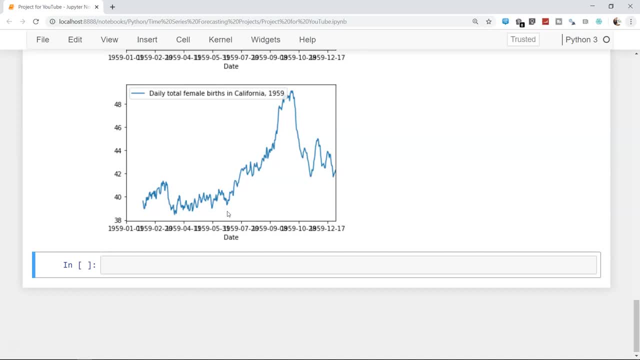 finding, at the end of this video, a confident confidence in you that yes, at least i can create the initial model, and with the upcoming video we will increase the complexities. for that the learning is easy. now what i want is to. what i want for you is to create a baseline model. so 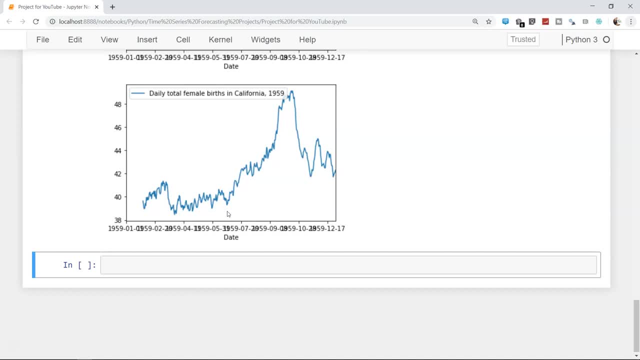 this is also generally the question within the interview, that what is a baseline model within the time series. so there are different types of models. one is a baseline model, i just said. there is a moving average model. there is an autoregressive model, there is an exponential model. 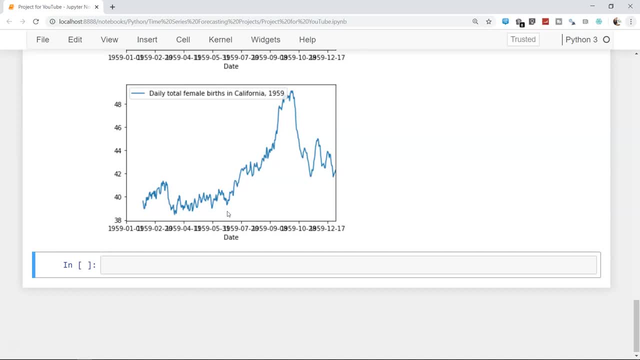 and there is something which is called as arema. there is s arema, which is seasonal arema. so you will see that as you will gradually increase, you know, increase your understanding about the time series, there are a lot of models, like i just said, but a baseline model is the model which helps. 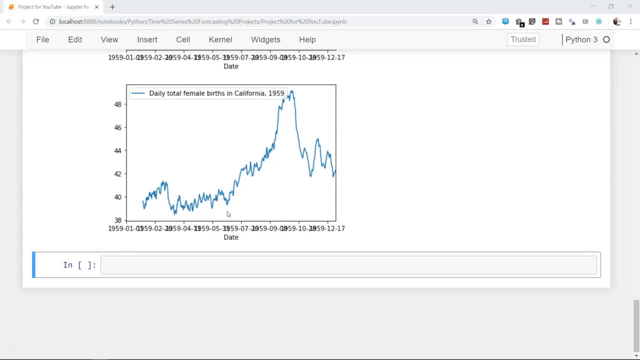 which is, first of all, very naive. that means very, very basic. its assumption is that your previous value that you have, so right now you know whatever day we are. let's say, uh, so today is 11th of november, so in 11th of november, let's say the, the date or the birth number is somewhere around. 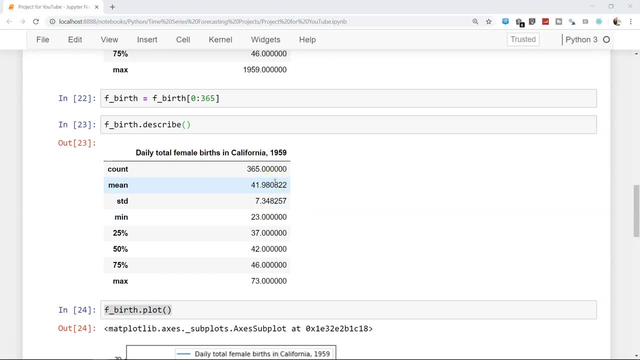 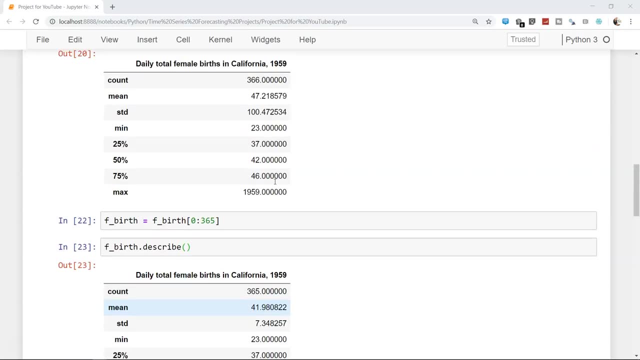 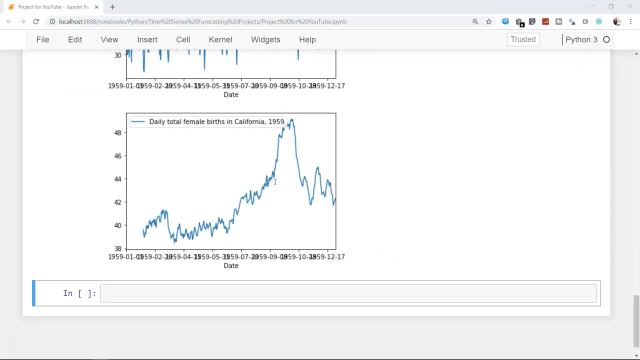 maybe 41. right, that means what we assume is tomorrow also, we will get the number 41. so that is what we are basically assuming with the baseline model. so history, the, the recent history, is the best reflection of the future. that's what the assumption is and, as you can see, 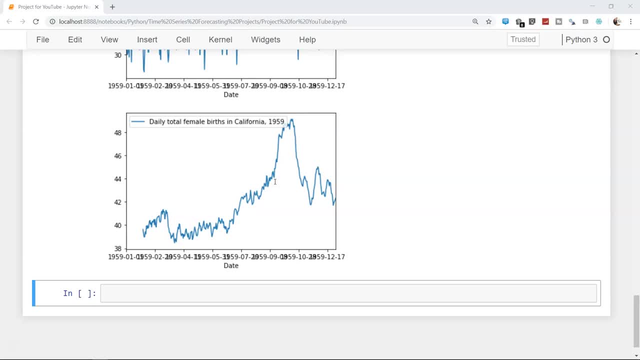 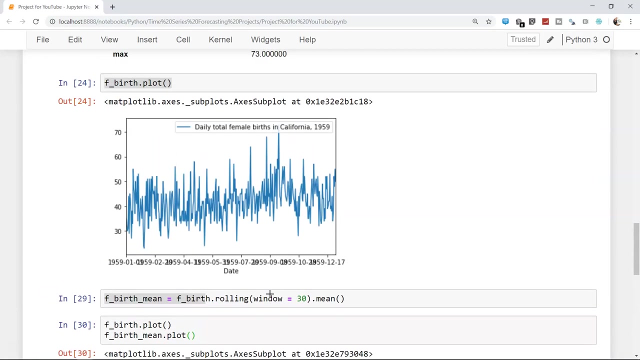 it's very easy: whatever your previous value is is getting used in the next value. uh, that's that's where you know you will create the baseline model and to create this it's very simple. so over here let me start with. so earlier we already had the values, if i remember, over here, 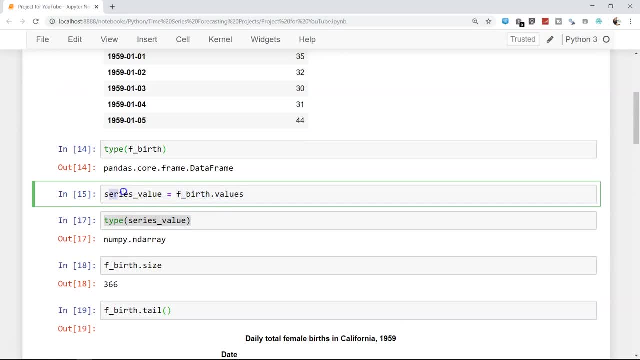 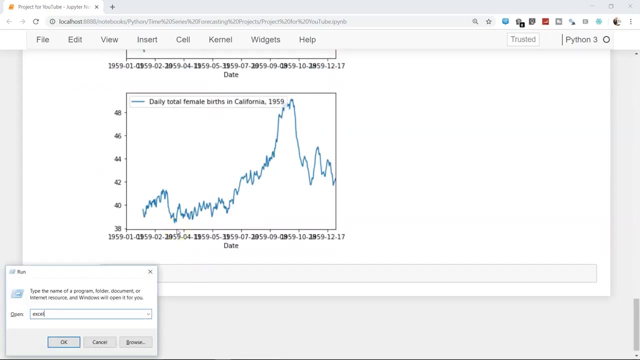 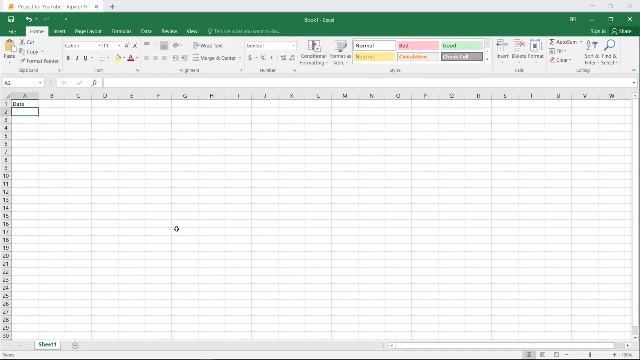 value f- birth underscore values, this statement. so, with this series value, what we will do is we will create one more value which will take the next value from the existing data series. so if i show you in excel, what does that mean, is so suppose, uh, this is date, this is a particular date for? 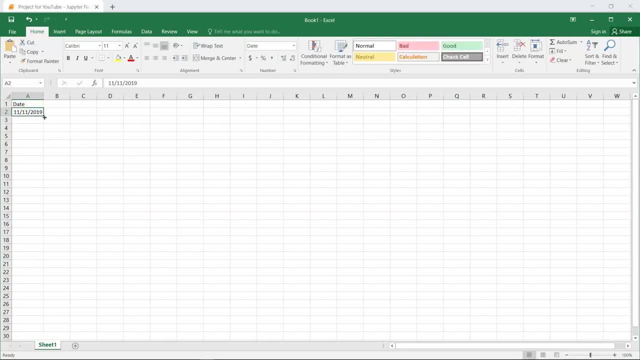 example this: and if we increase, let's say this is what it is, then right now, if it is 41, and tomorrow 45, and then, uh, 40 and then 38 and 41, let's see this is how our series is currently. so series t plus 1: what will be? so this 41 will? 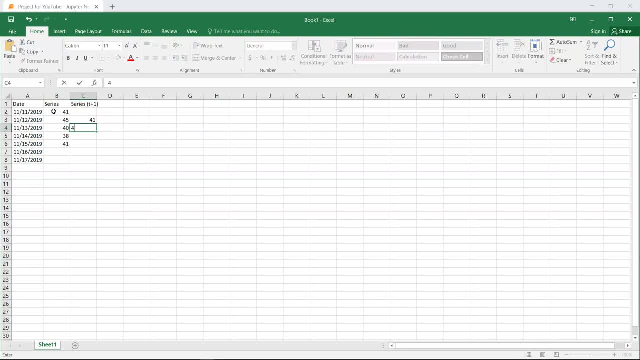 come over here. 45 will come over here, 40 will come over here. right, so, as you can see, this is how the values are coming. as i said, what we assume is the previous value is the best reflection of the future and, as you can clearly see, this is the actual value. this is the predicted. 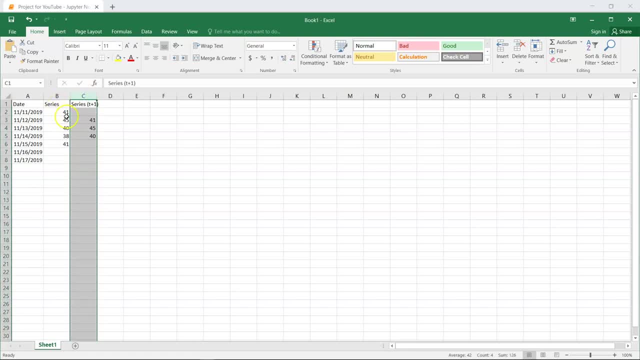 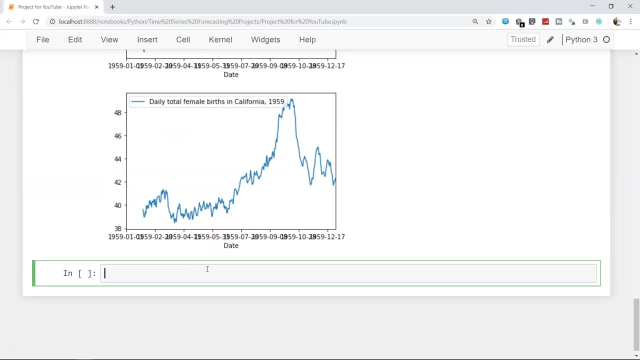 value. predicted value is nothing but the. whatever our previous value were, we were taking it for the current value. so let me go back. so this is what we were going to do, so series underscore value we already had. so what i create is birth underscore, df data frame and pd dot. concat, concat, yeah, so concatenation function, basically. 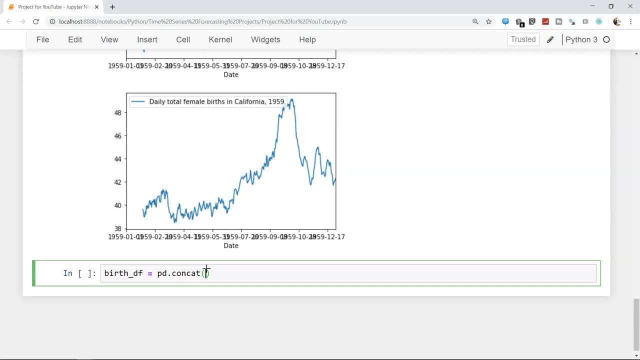 takes two series and create one data frame. so one series we already have, that is series underscore value, but we need to create one series which is taking one more value. so first of all we have series underscore value, that is our current series, and then we have series dot values, dot shift method, shi, ft, shift by. 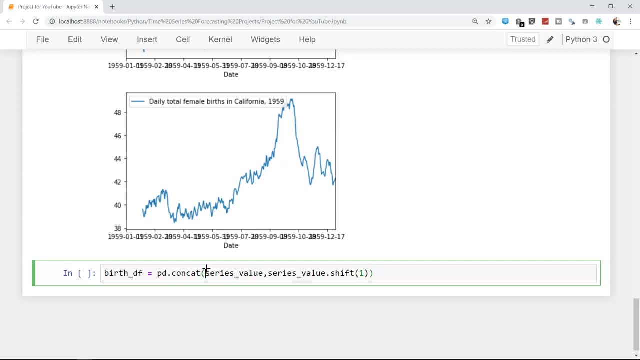 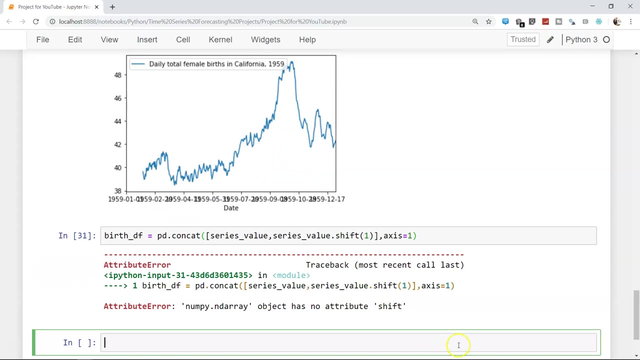 one place, right? so the excel manual operation that we did, we did it over here and surrounding it by: because this, this is part of one data frame and axis equals to one. because we wanted columns, we execute this all right. uh, number of values we have here is one and we need to create one. 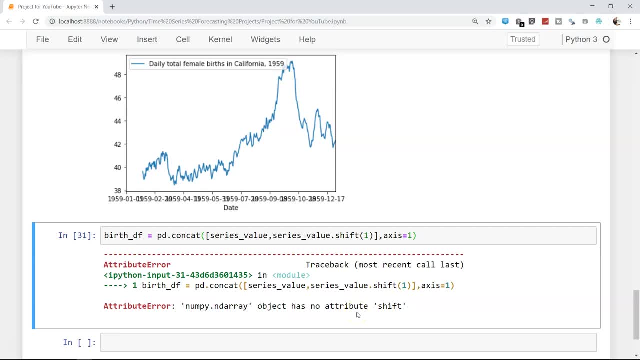 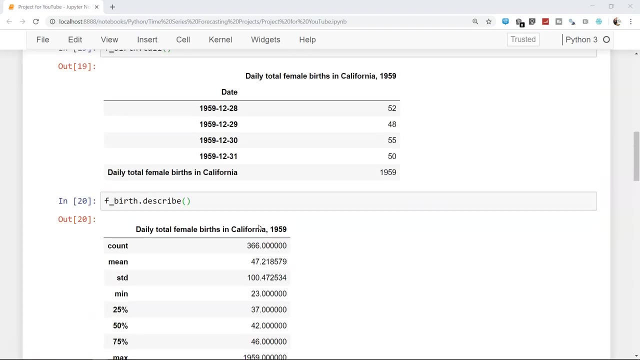 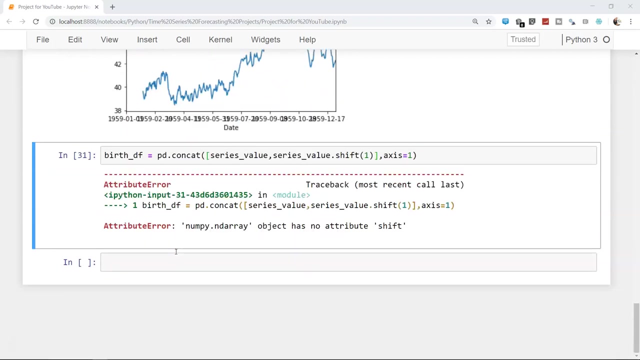 by array and the array has no attribute as shift. all right, so what do we need over here is: so this shift is part of the pandas uh function or the pandas library. so what do we need is, first of all, the data frame f underscore path, right, f series underscore value. so what i can do is i can just 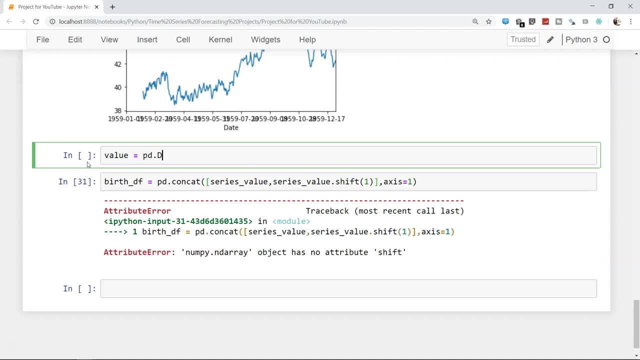 create something like value pd dot concat and then i can just create something like value pd dot data frame. so pd dot data frame is nothing, but it's a function part of the library which will correct, connect- uh sorry, convert- a series into a data frame. that is what the requirement over here. 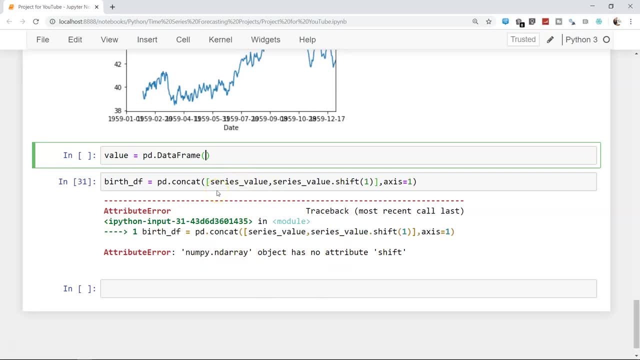 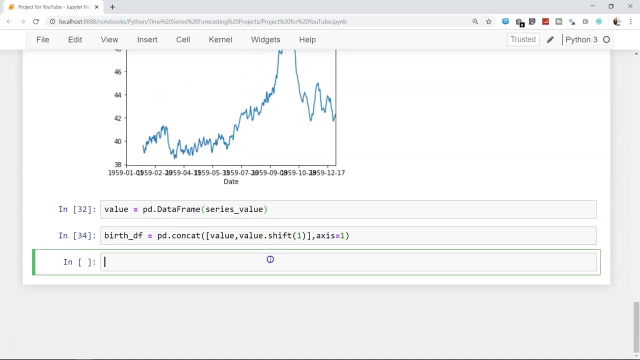 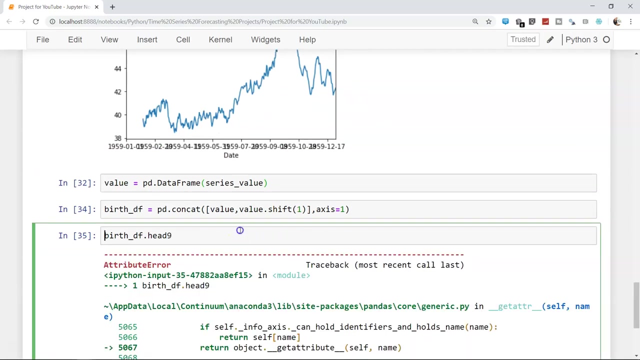 because it's it's not part of numpy array. so what do we need? is uh, series value, right, series underscore value. so now series value and everything. uh, sorry, value. i will remove this value value and now everything is fine. so birth underscore: df, dot hat, oops, had. 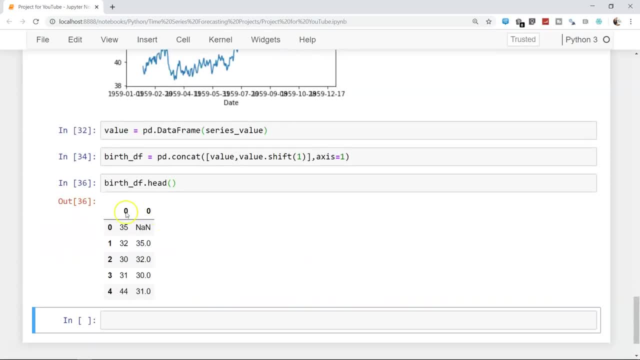 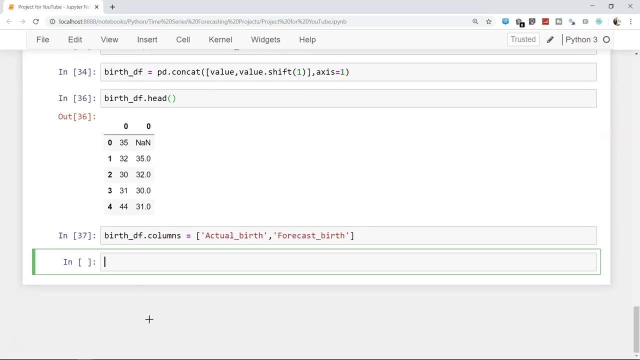 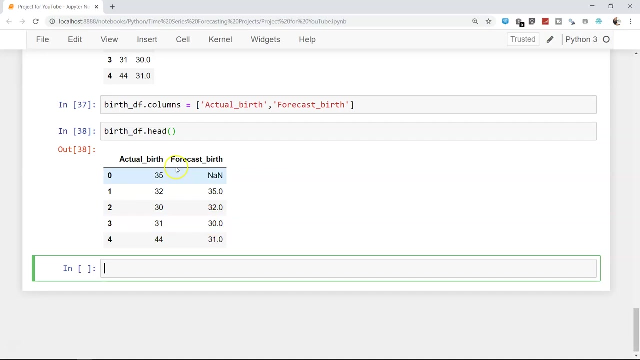 we have to give the headers to it, right. so birth underscore df dot columns and within the columns. so here equals to basically, and t, t plus one or whatever current underscore birth or something like actual birth, which is much more clearer, and for a cast birth, that is it right. birth underscore df dot head. and this is what your value is: actual birth. 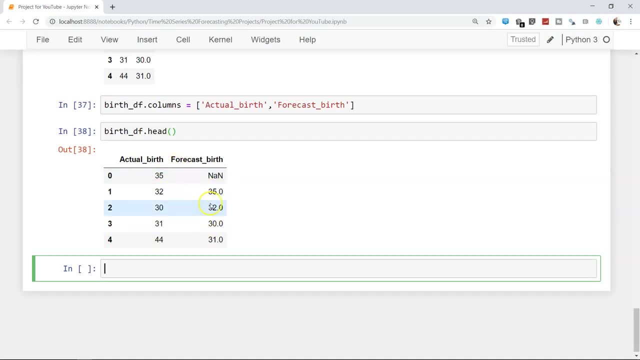 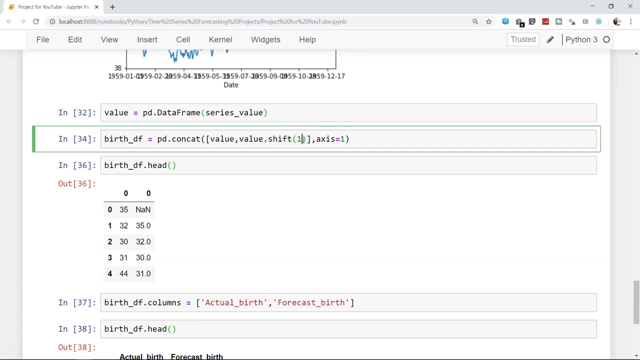 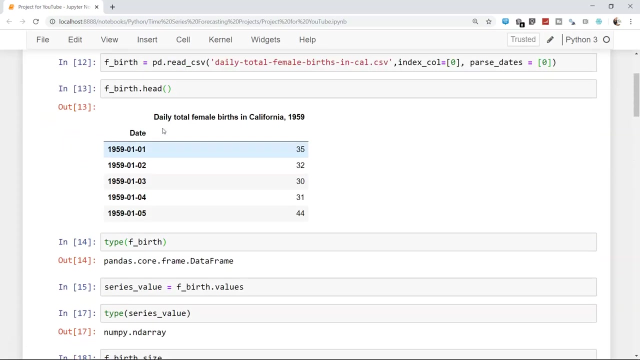 for a casted birth. so 35 is coming over here, 32 is coming over here, 30 is coming over here because we have used the shift function over here. so this is one thing, one way of doing it. another, very straightforward way could have been using directly the. 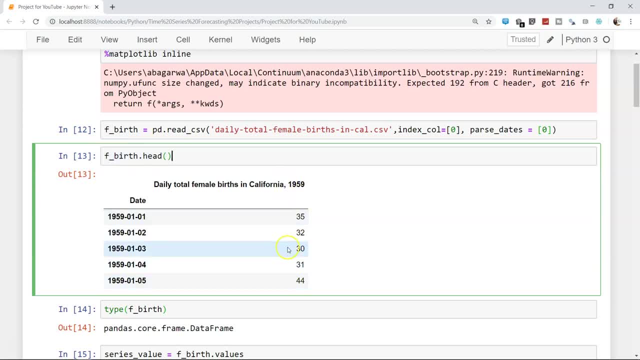 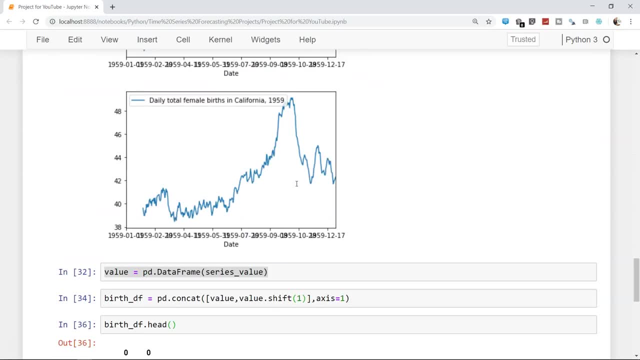 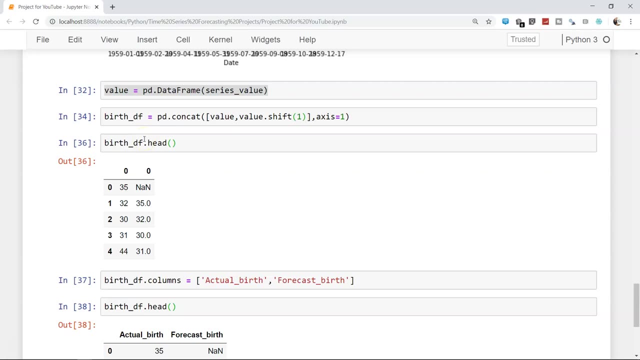 f underscore birth over. here we already have this column. we would have just used the this particular column, dot shift and that would have resulted into the this, this particular matter, so that as part of exercise, you can take right that from here we have converted the data series into a data frame and then use the shift function. however, we had the 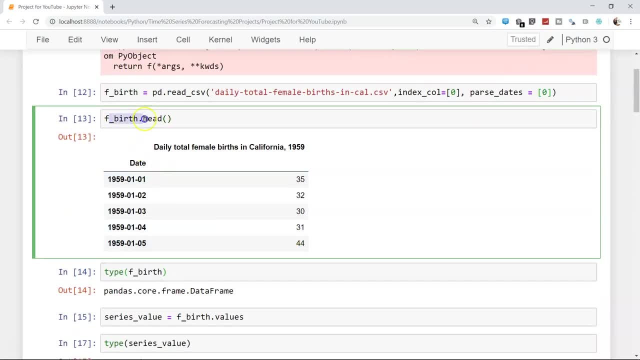 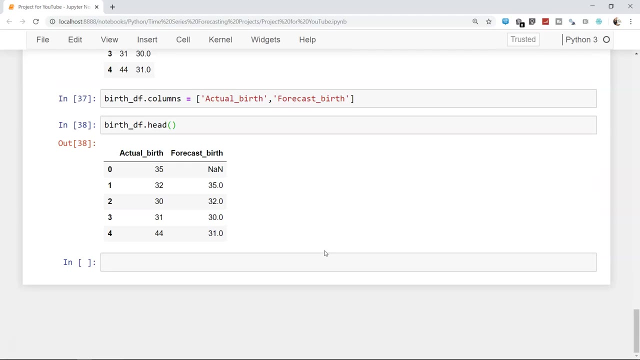 functionality available already, because f- underscore birth is already part of the, the data frame and we could have directly used the shift function on this. so how you can do that, you need to show me by doing it and i will put this particular, uh, this particular python notebook. 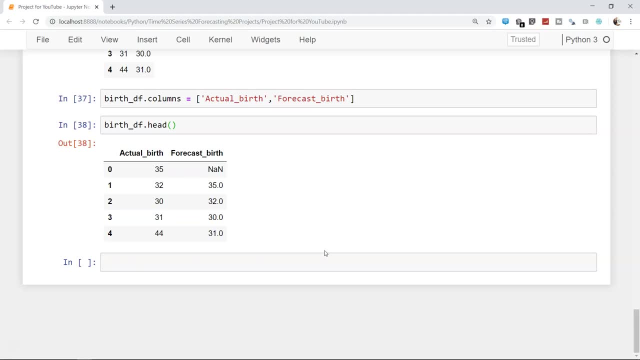 uh, in my description, and then you can go ahead and directly use it, right. all right, so you, after this, once we have done this, is to identify the error that is present. so there are two ways to figure out the error. one is either you can figure it out on the complete 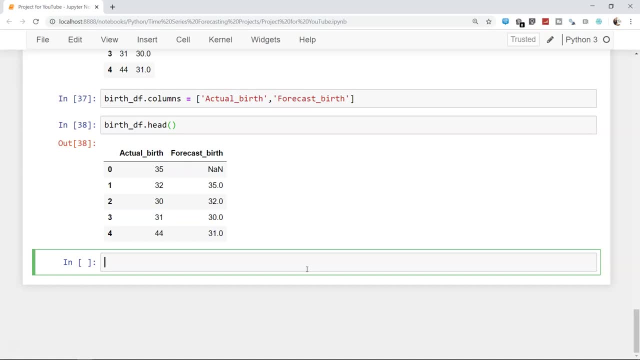 data set, or you can have the train test. so in this case, train test really doesn't make any sense because this is a naive model. the previous value is being used on the current value. so i can show you both the approaches, but up to you how you want to decide. if the data set is small, like 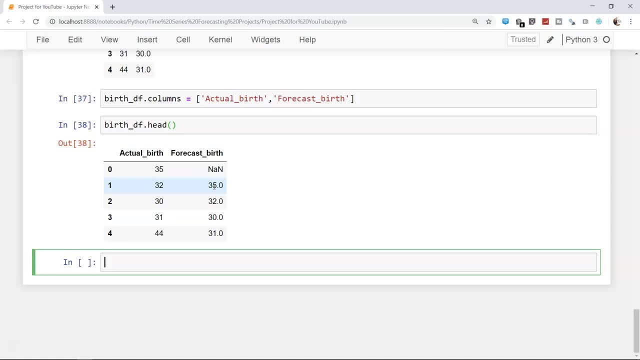 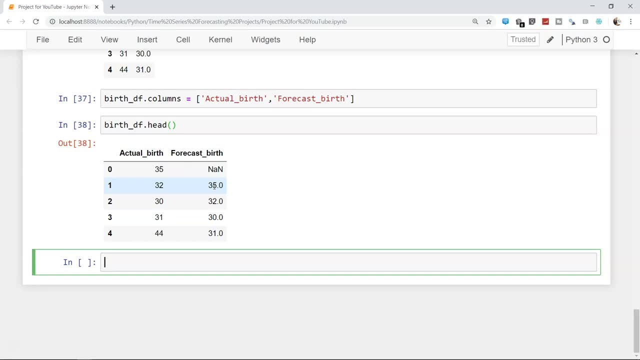 a partial data by doing some sampling or directly taking it, and then you know, go ahead and use it. the error, so how you can, or calculate the error. so how you can calculate the error is by importing the, the mean squared error module. so from sklearn dot matrix. 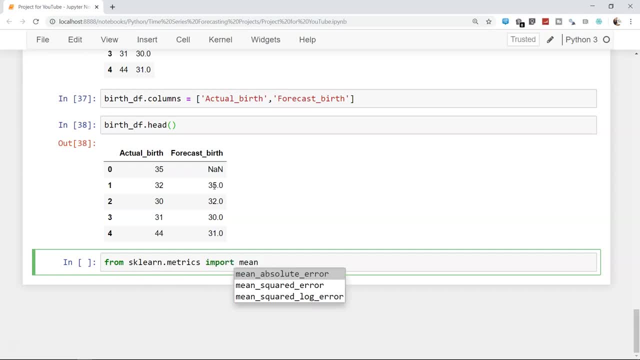 import mean squared error. i have just pressed tab mean squared error and i need to import numpy as np because i want to take a square root of mean squared error so that because mean squared error will going to square, do the square of the current value. that means if the 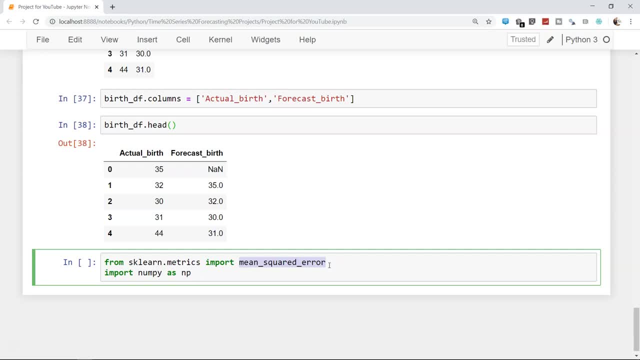 mean square mean value is 10, the square value will be 100. that is not interpretable, right? but if we take a square root, the, the square root of 100 will be 10. then the mean error will be 10. so 10 is nothing but your actual birth value. that means you have an error of 10 birth values. 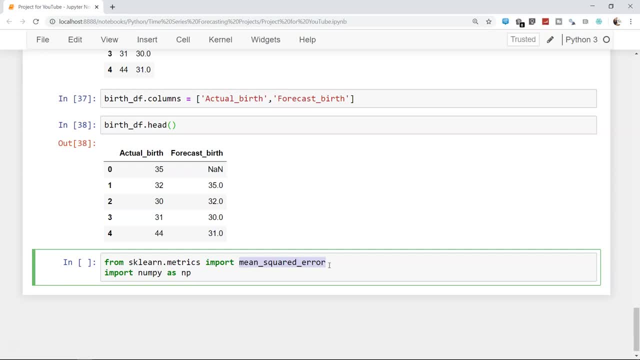 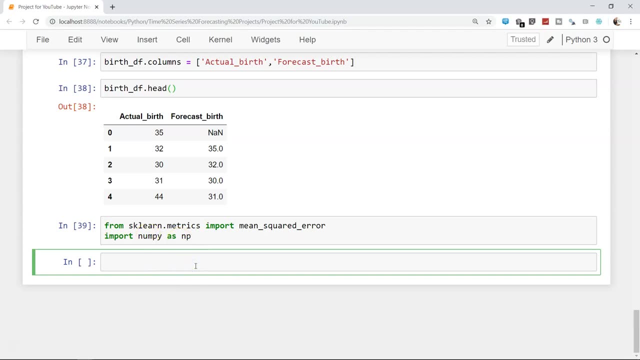 which are present in the data set, which is nothing but the part of the variation. so that's why i'm importing the numpy as np and to calculate the error. so birth underscore error equals to mean squared error and the actual birth value. so here it will be. 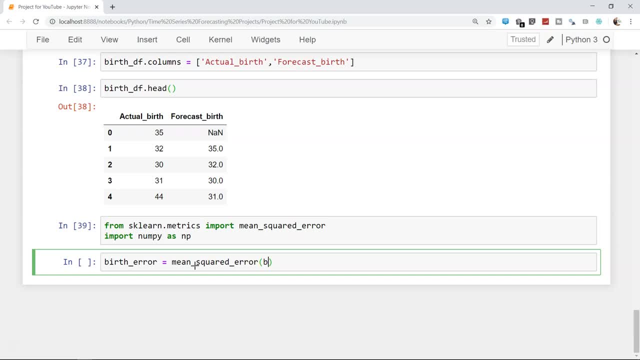 birth underscore df- thought actual birth comma. birth underscore df- thought for a cost. but now this will return an error and the reason: if you see this data, the first value is not unrecognized for the else value, which is 22, 2 b df, dot b does not matter. now i have to write error, what i am going to do here. 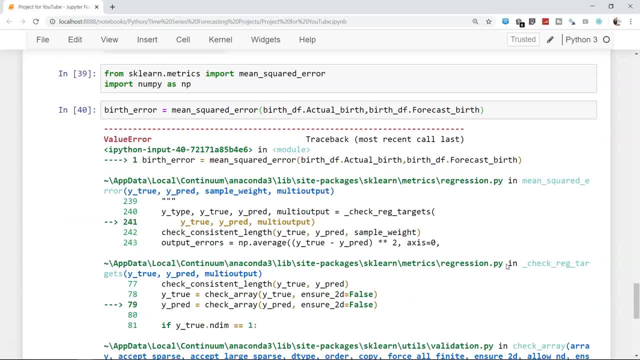 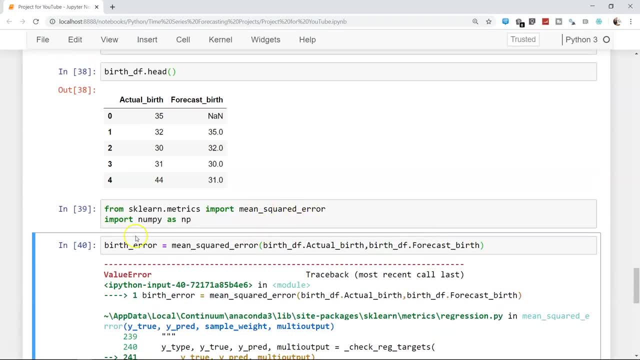 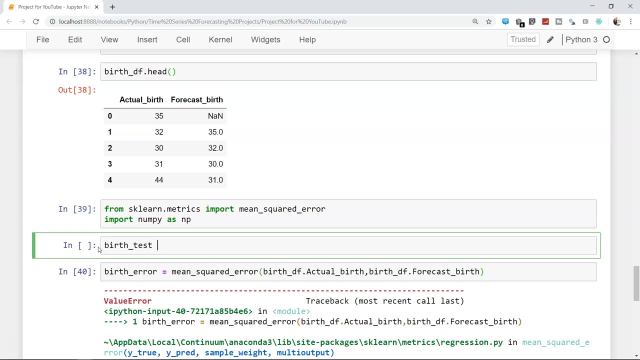 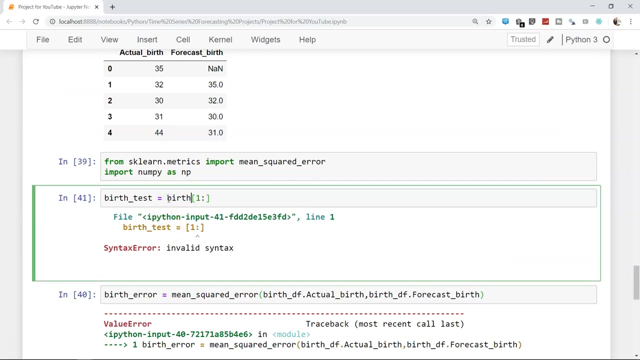 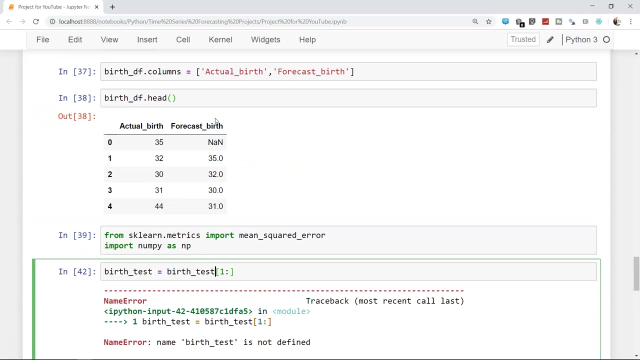 number, that means the missing value. so if I just go ahead and execute, it contains any end right. so you need to remove this over here. so birth underscore test equals to take it from the one one is nothing but this one till end. that is what I'm saying. so if I execute over here, birth underscore- yes, I'm fine now. 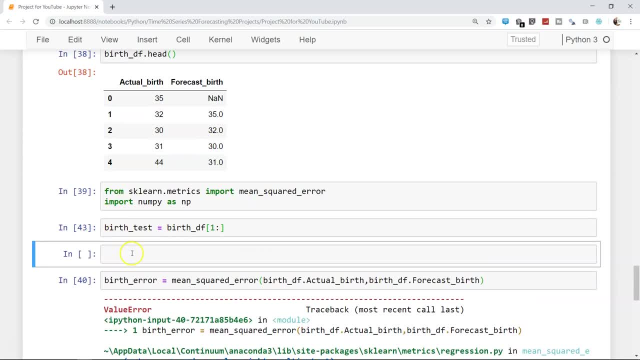 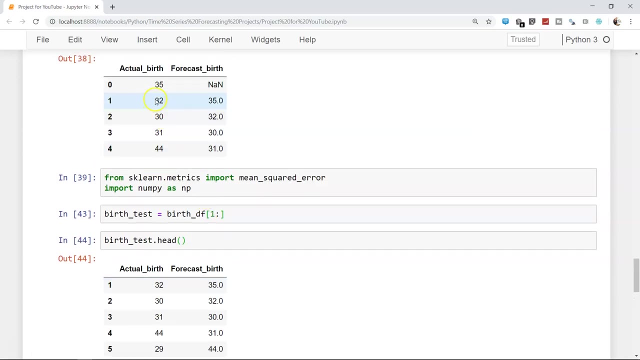 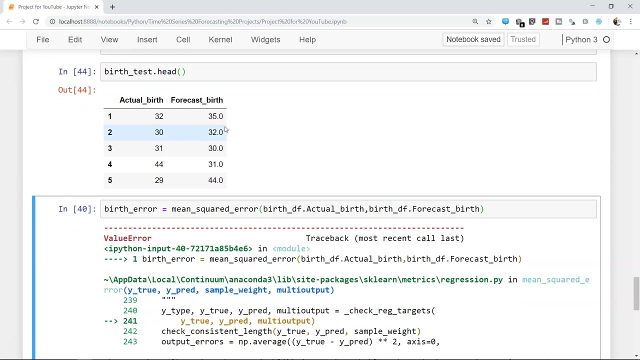 and if I press B, which is creating the cell, what I want, just to test it: birth underscore test dot head, I have this proper value. so now, if you see, it is coming here from 32 to 35, 30, 30, 30, 30, 30. okay, we have removed the first. now this is basically our data set. 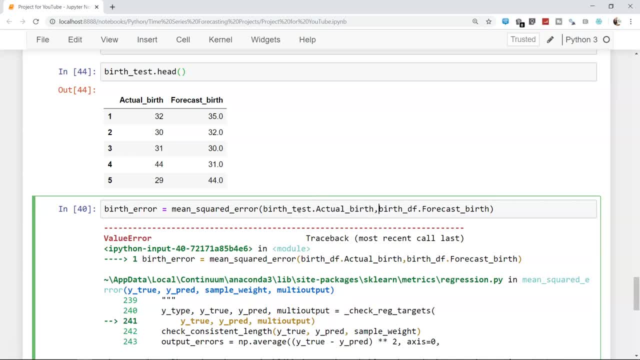 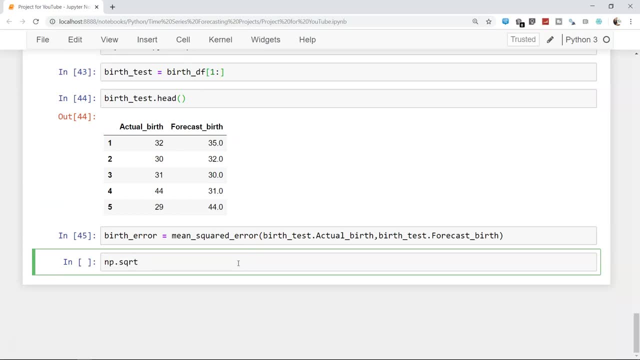 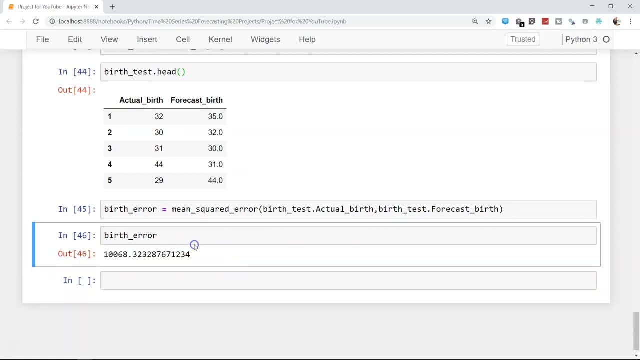 so we will say: birth underscore, test birth, let's go test. and NP dot sqrt. so let me first show you the birth error itself, which is a mean squared error. so one, zero, zero, six, eight doesn't make sense, right? so what we'll do is NP dot sqrt, birth underscore error, and that is. 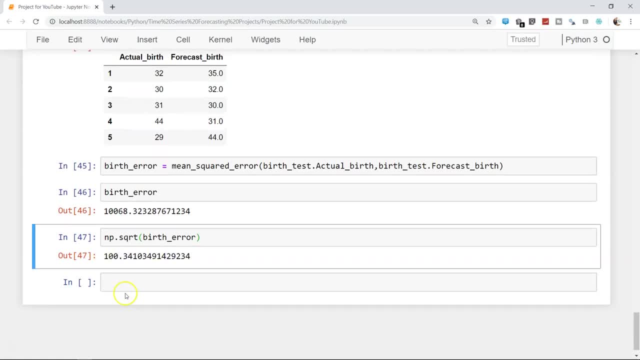 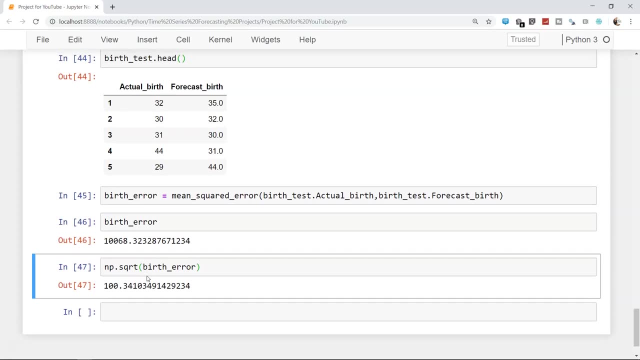 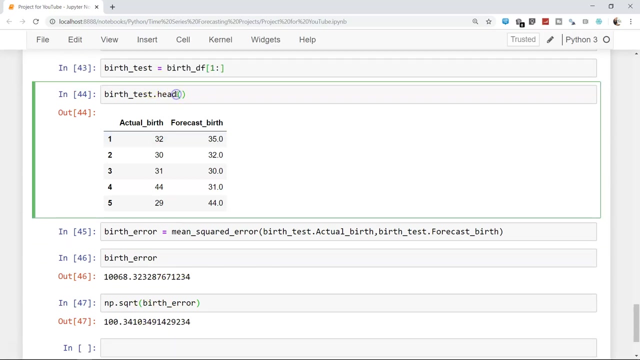 hundred. so again, you know, doesn't make a lot of you know sense, because hundred is definitely too high, but this is something which you can say become a baseline model and before I confirm on this, what I want is just to check the tail on. so I want to make sure yeah. 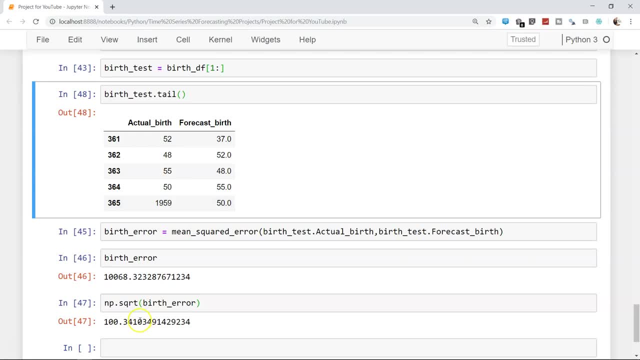 that's why I was thinking 1959 is coming right, that's my hundred- was not making sense for me, and because of this 1959, if you remember, the hundred was coming as part of the standard deviation and that there also I said it's, it's incorrect. so 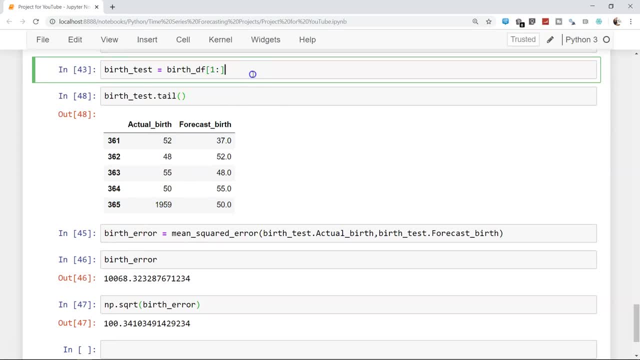 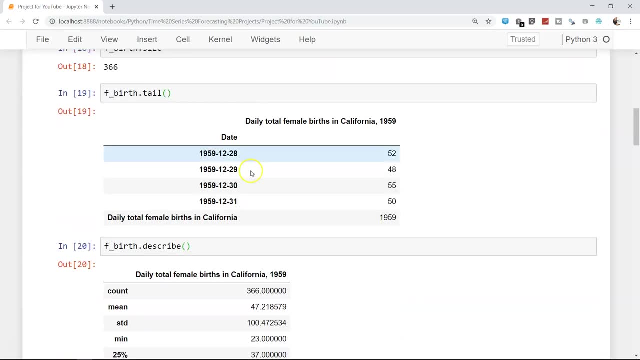 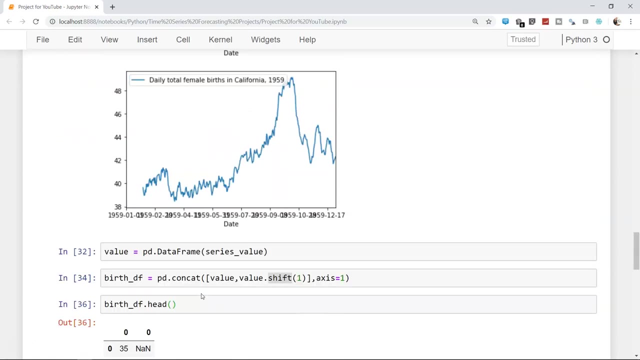 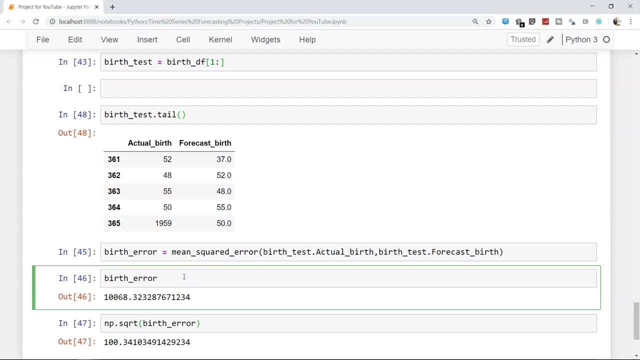 we need to remove this, this particular row, so once we have done this, so if you remember what we have done earlier in case of a data frame, when we had described it- 0, 2, 3, 65, right. so here, but underscore test, we have this 959, so we. 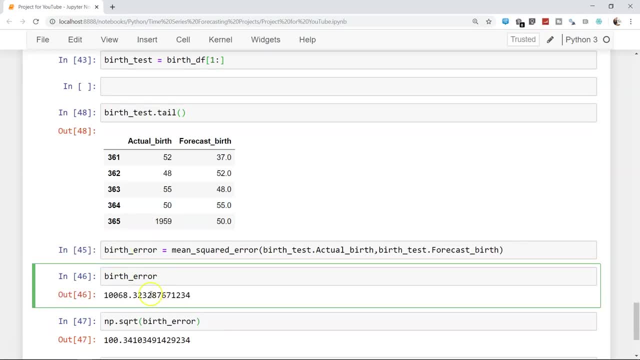 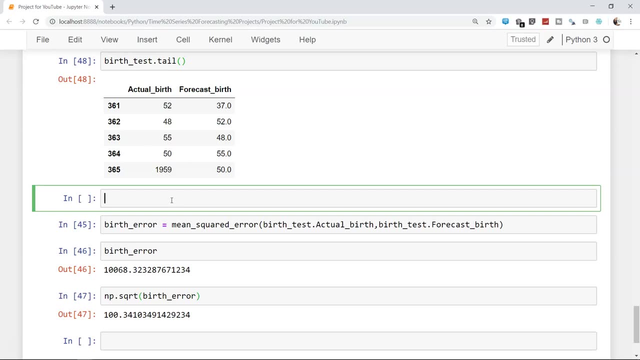 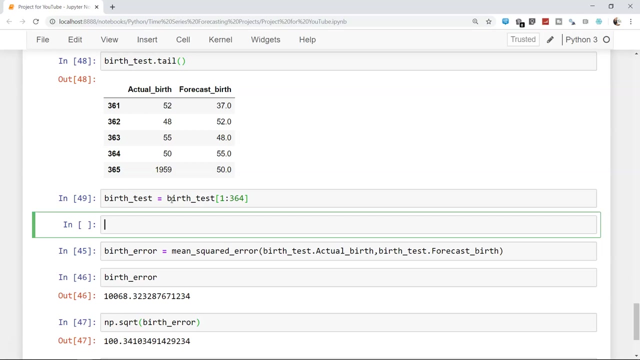 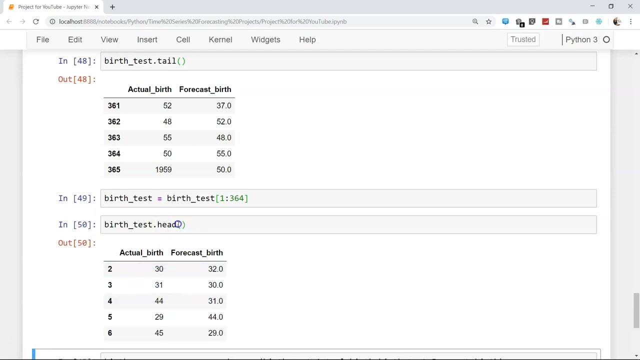 have to take two 364. so over here before this, press a and. but underscore test equals to birth underscore test and from here we will just take from one to three. sixty-four. we do that. So this is. this has come from 2 and we have removed the first value. so what I need is: 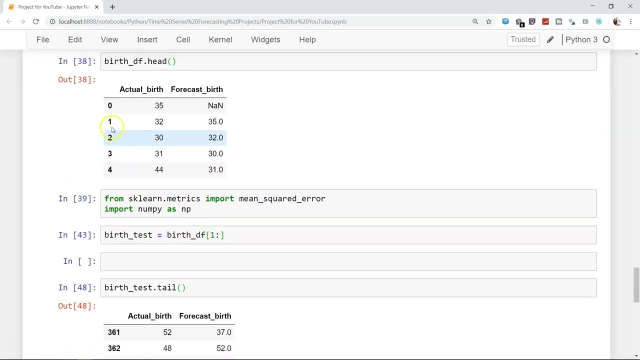 basically from this, this has actually become 0 in the from the perspective of index. So 32, 35 and 30 and 32.. Right now what we are getting is 30 and 32.. So, accidentally, what we have done is remove this as well. 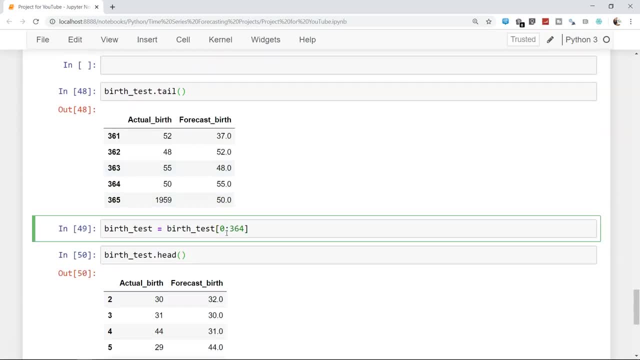 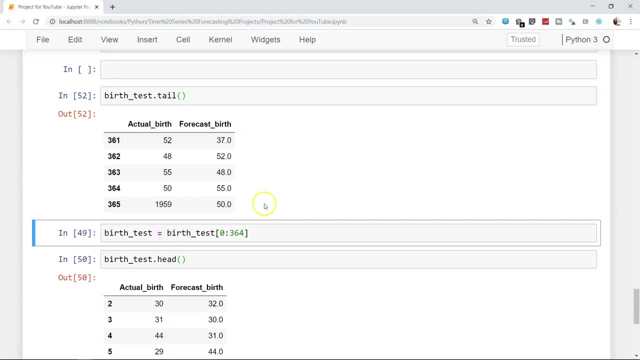 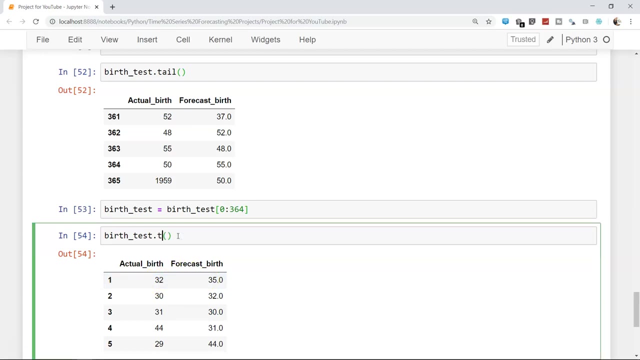 Ideally, what I should have done is 0 to 364, and to do that I just need to run this again: Birthdf. tail is coming from here and birth as this head. now I am fine. 32,, 30,, 34 and. 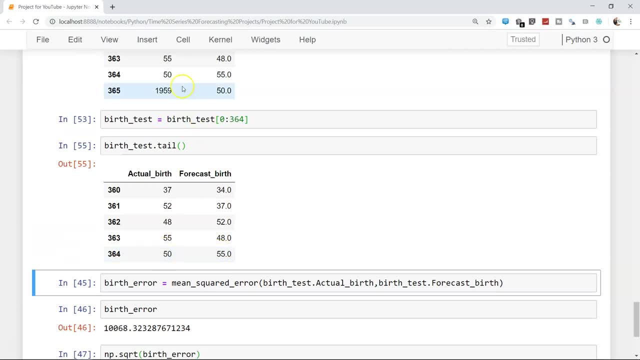 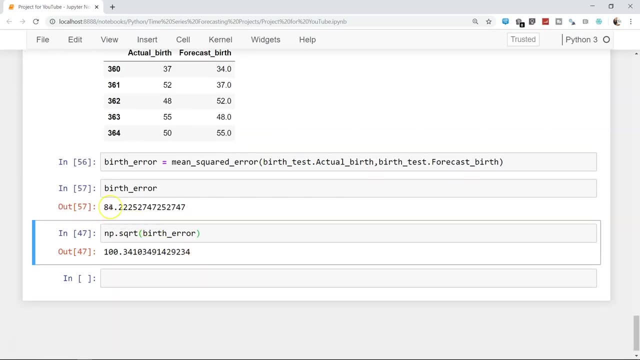 tail is over here, yeah, So this particular observation, as you can see, is removed: 50 to 55. and now, if I come back here, See I have removed the birth error, which is 84 from 10,000. it has reduced to 84.. 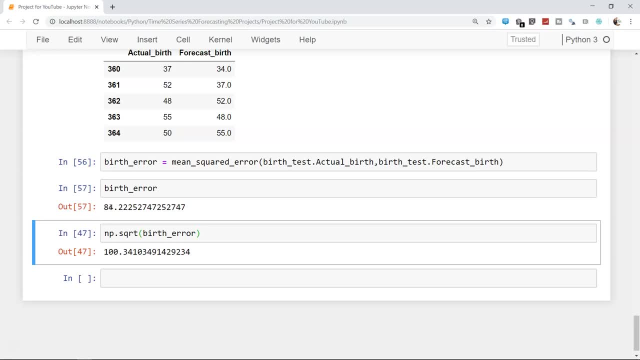 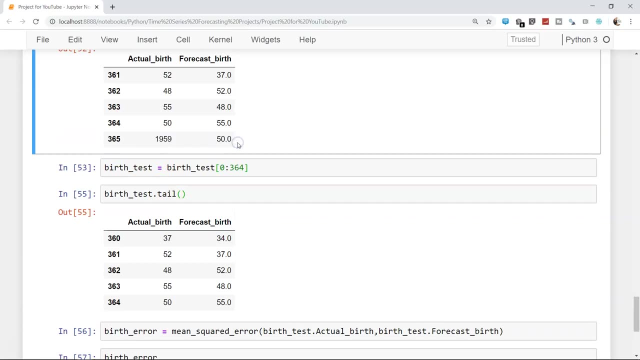 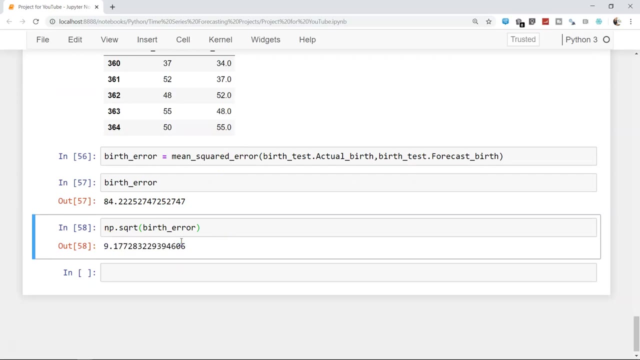 You can see, that's a significant improvement, and that is only because we have to make sure that we know what are the outliers. that is present right. And now, if I take a square root, it's just 9.177,. that means that is an error of 9, right. 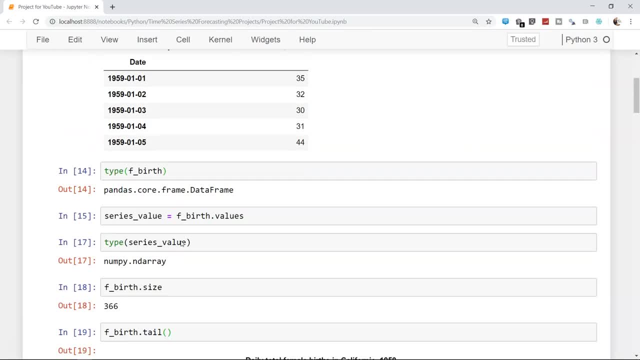 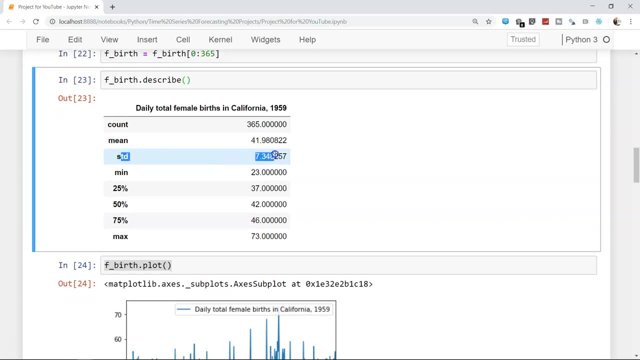 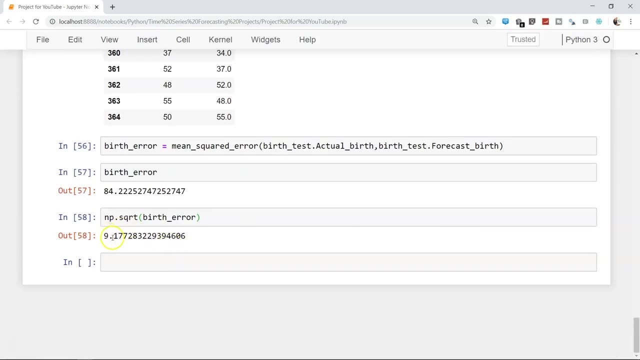 And if I go above and see the describe method over here, standard deviation is 7.. So without even you know going to a model like this with the help of standard deviation, from that also you can see that the variation is 7.. 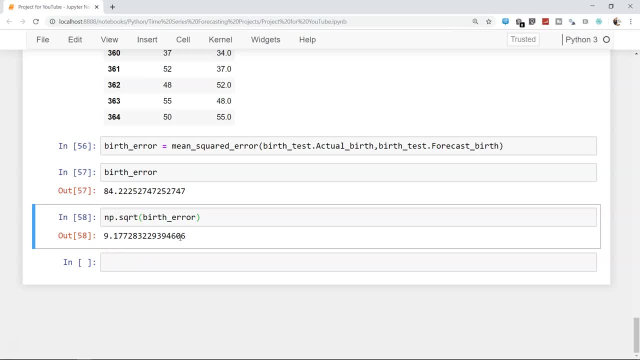 But with this you can actually see, when you are using the naive model, what is the error. So 9.177 has become your baseline. That means this is such a basic technique and with that technique we can get an error of 9 birth of every day. 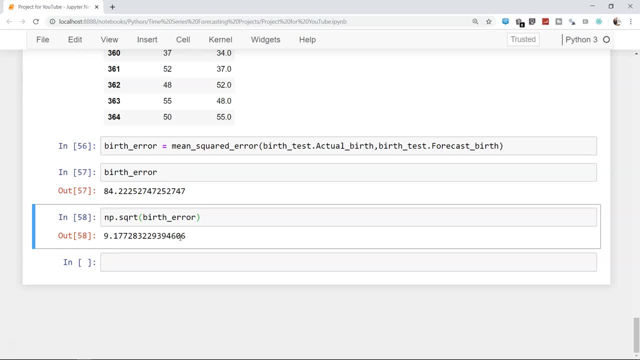 That means there may be a plus minus of 9 birth error. that can happen in your prediction. So what does that reflect? This reflects that whatever advanced model you are going to produce- for example, if let's say you take exponential or moving average or autoregressive or the ARIMA, your model- 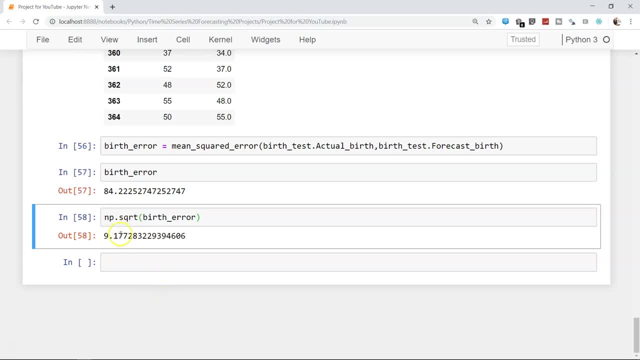 should always have the value which is 9.177.. That is, below to this value. That means the error should go down as much as possible. So, as I said, there are many models, but finally, in any case, we come down to something which. 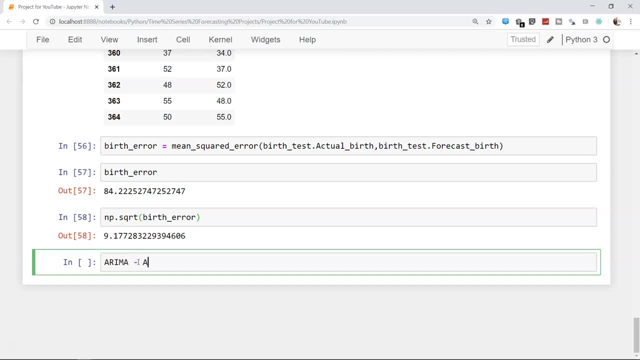 is called ARIMA, right, ARIMA is nothing but Autoregressive, Integrated Moving Average. So what it does, It has basically three components: One is autoregressive, right, Then you have integrated and then you have moving average. I told you, moving average is nothing but the smoothing part. 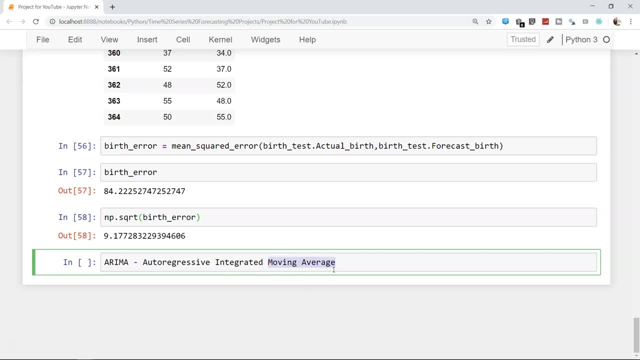 You know how you smooth by removing the errors or noise from the data and see how good the value is. Autoregressive is nothing but what it assumes is. the previous value is correlated, the current value is correlated with the previous value and the previous value is the best reflection. 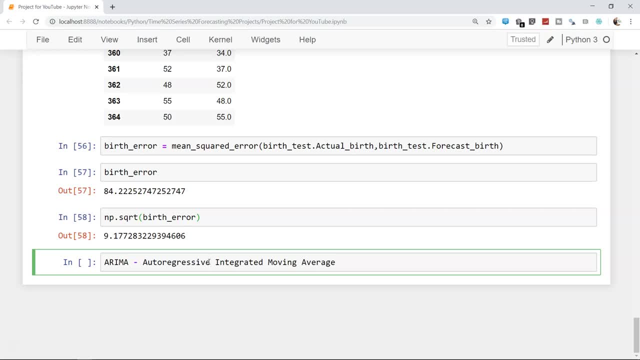 of the current value. So we see how well the values are related to each other, and integrated is nothing but the order of difference. So, for example, like I said initially, that your series or your time series should be stationary and to have the stationary time series you need to perform some operation. 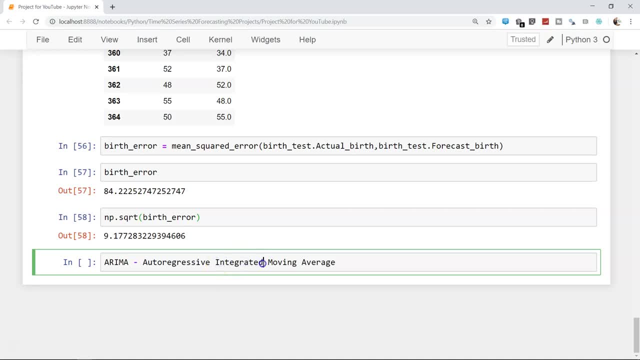 And this is basically the order of difference, This is basically the this, this operation, which is which it says integrated. So integrated is nothing but the parameter D, if I just mentioned. And to better understand this, what I can do is come to the Excel or, instead of opening, 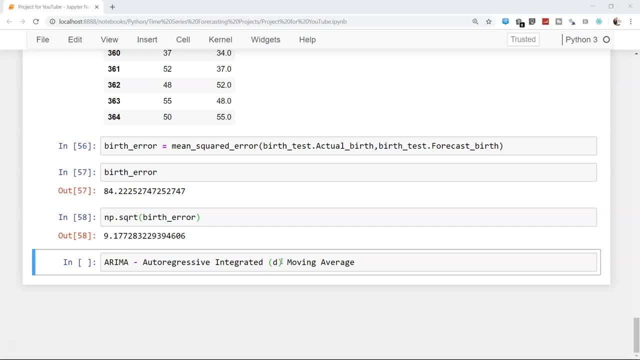 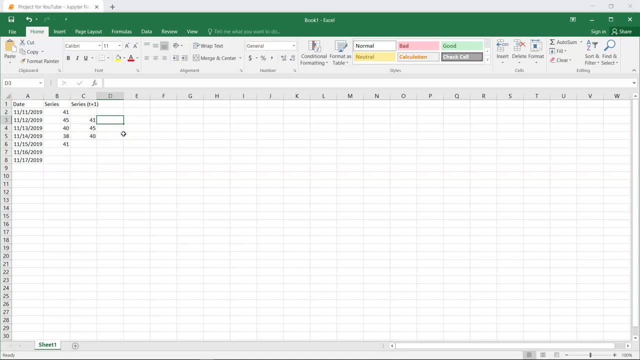 a new Excel. let me open up the previous Excel file that we created. So what it does is basically figure out a difference. So, for example, we are here, So this minus this, then it's a series like this: if that's a here, you have 35.. 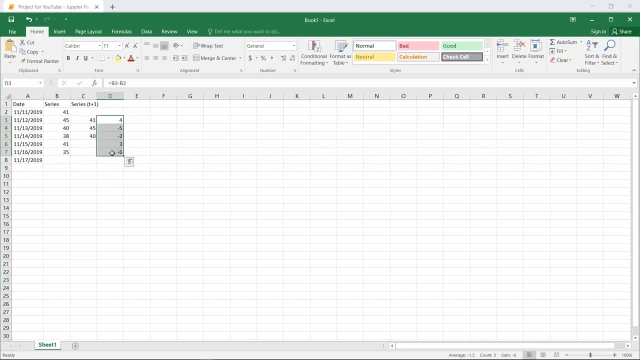 So, with the help of this, what it tried to do is remove the, remove the error wherever it is present in the data set and try to create it a see the, the stationary series. that means So there is a seasonal component, there is a trend component, all of that. 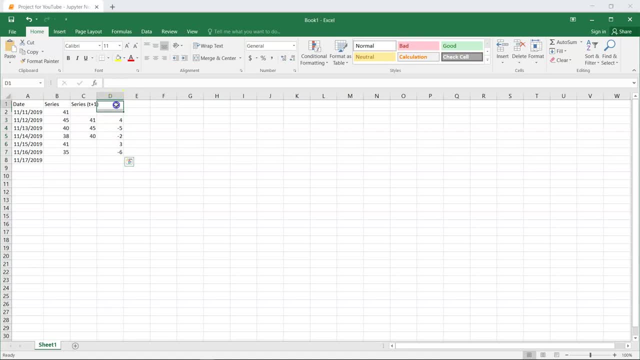 It tries to remove that And this is the order one. So the value of D will be one in that case. So order equals to one. that means D equals to one or D, and that's how you will specify its value. If you want the two order difference, that means D equals to two. 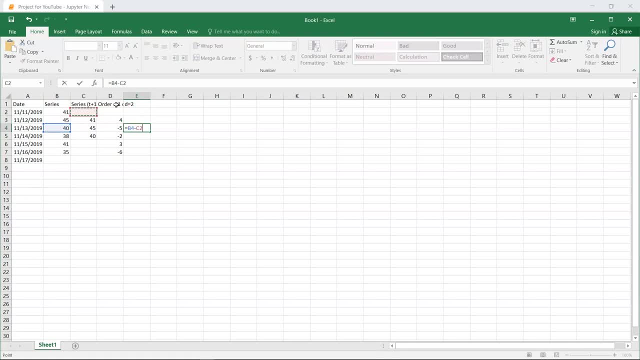 What you have is this: you are on second instance and going back to the first instance, Then You are just dragging it down, right. So this is D equals to two. Similarly, you can have D equals to three. So generally I have not seen going beyond to two by generally, by zero or one we are. 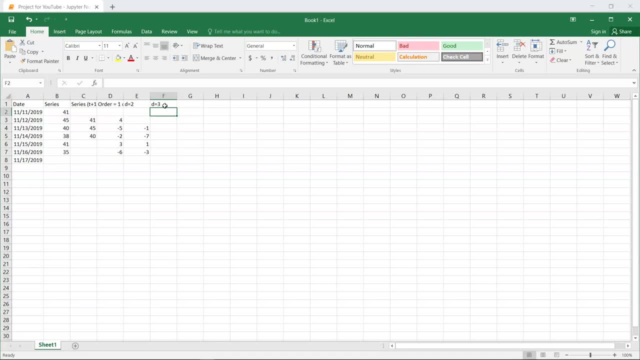 pretty much done And in some cases we can even go to two, but I have never seen we are going to a level of three. So zero, one or two is something you can experiment with. it right. So coming back to to this, 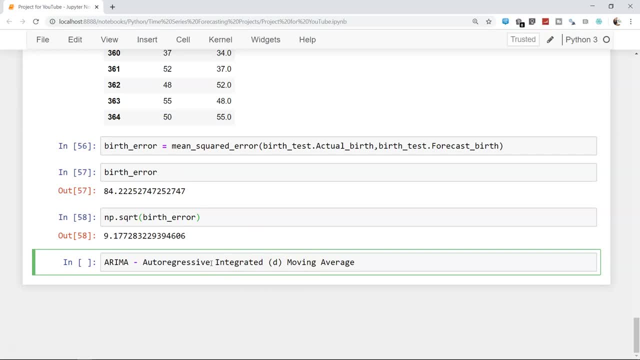 Autoregressive. like I said you, you have a way by which you can identify its value. So it's a value of P and a moving average is nothing but the value of Q. So autoregressive for autoregressive and moving average. 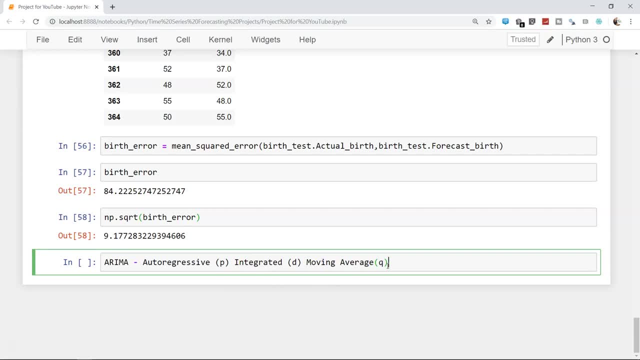 What we have is basically ACF and PACF curve, which is autocorrelation, and partial autocorrelation, which checks from uh, from the current, how well the current value is correlated with the previous value And when we see the correlation is present, is not present after the first value or second. 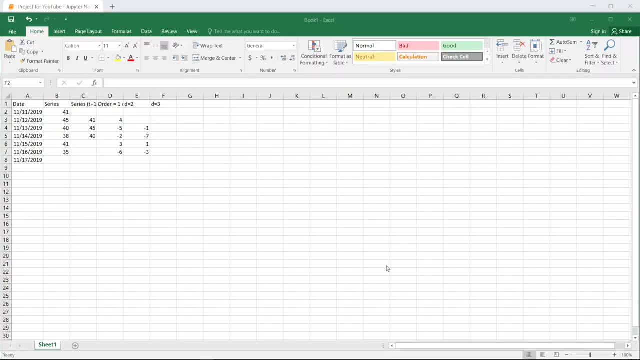 value, then we go ahead and use its value. So what I mean by that is: I'm over here, I am creating one column over here, insert. So this value somehow will be correlated with this. This value will be correlated with this. 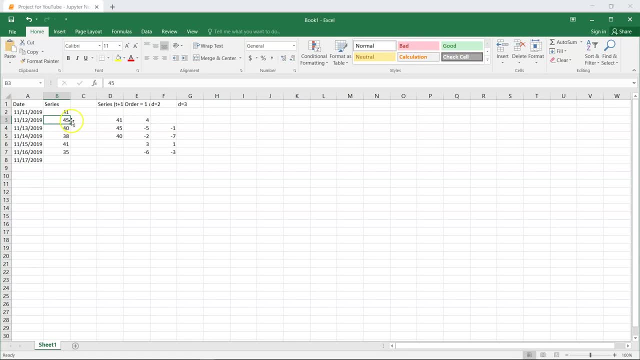 If the correlation is present, that means this is the order of one. we will not take it. Correlation basically, uh creates a problem or in try to influence it, And we just want a very normal model which can work on any- uh you know- scenario which. 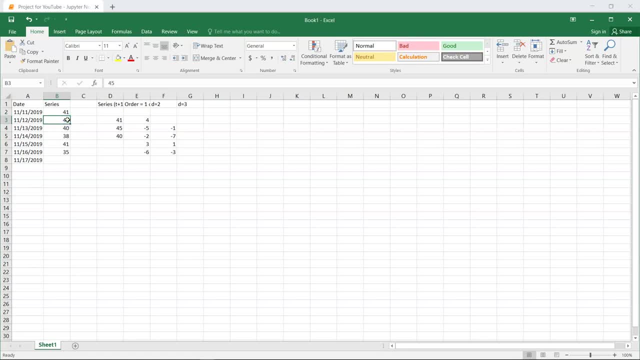 it may face in the future. So we see that at level one there is a correlation present, So we move ahead. When we took at level two, that means 40 checking, 40 is correlated with 41,, 38 is correlated with 45.. 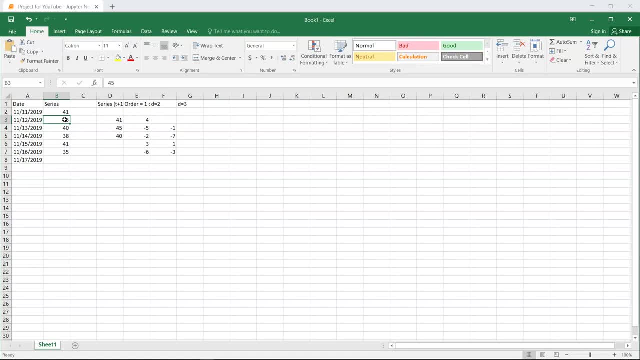 That is P value equals to two. Okay, That means on level two, you know there is the correlation. If it is not present, we will take P equals to two. If the correlation is present at level two, we will not take it. 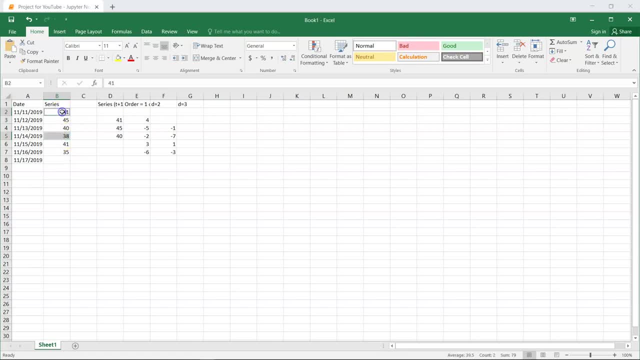 And then we will move on to the third. So we'll check 38 with 41,, 41 with 45. And generally at level three. by level three you are pretty much there and, uh, you would go ahead and use it. 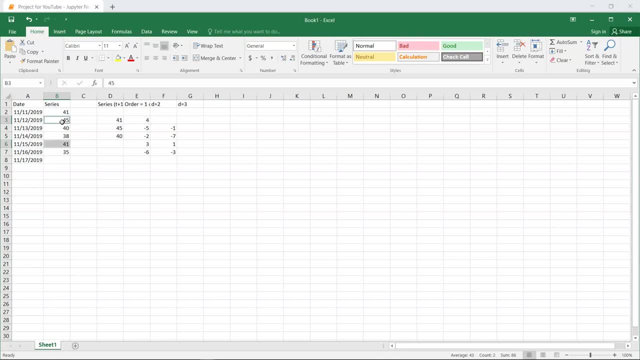 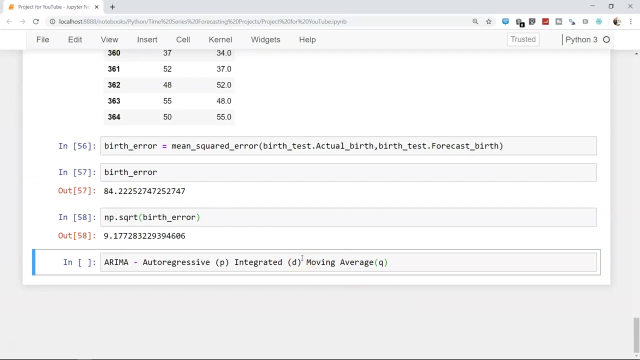 But that completely, completely depends on the data set, about how your data set is distributed. Okay, I mean even going to an order of three or four or five in this case. So let's go ahead and see this, uh, how you can create the, the uh, partial autocorrelation. 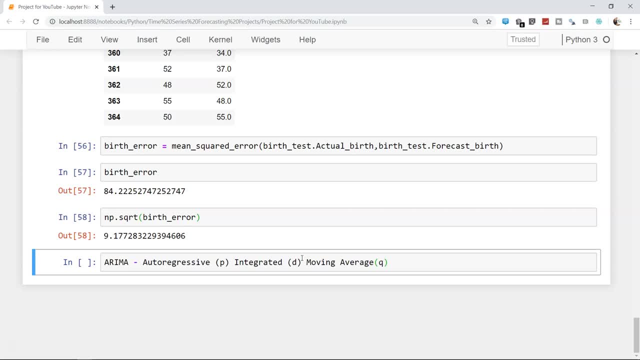 and uh autocorrelation chart. For that I will press B to create a new line. So from so the package we were going to use this: stats, models, dot graphics, right, And then the T, S, A plots: import plot underscore ACF. plot underscore P, A, C, F. execute this. 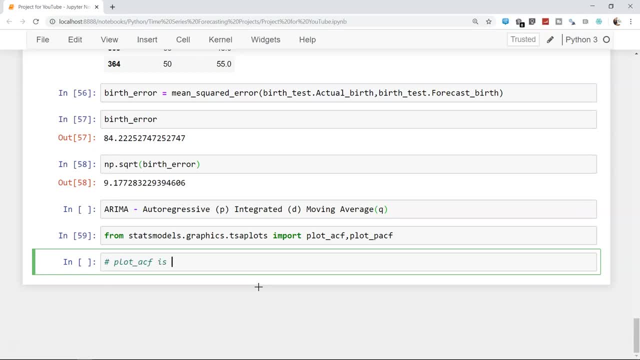 So I will say: plot underscore ACF is to identify parameter Q. That means you have something like a model. Okay, So what we will be using is Arima PDQ. So D value is somewhere around zero, because we have seen initially from the graph that 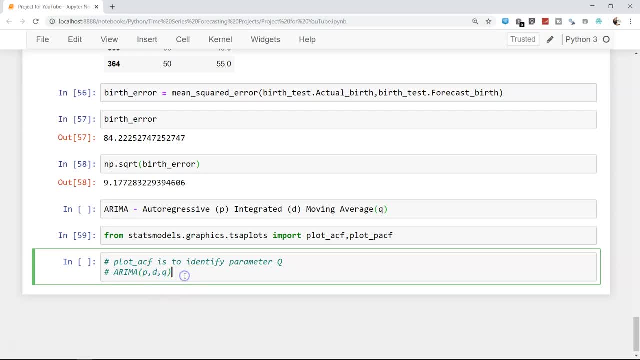 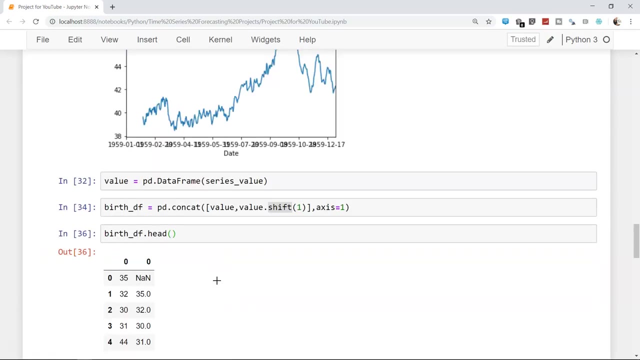 the that it is a stationary. So PDQ is this Q value we will going to identify with the help of plot underscore ACF. So let's go ahead and see. So plot underscore ACF. And what was the name here? Okay, 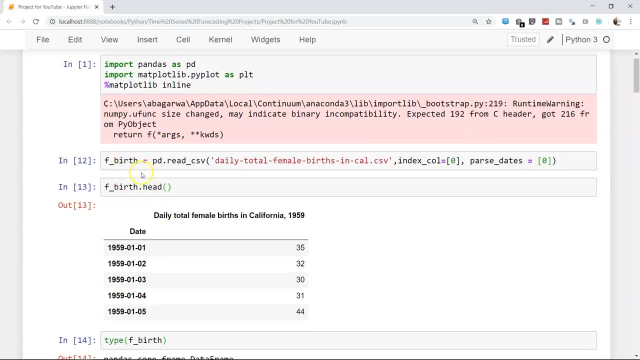 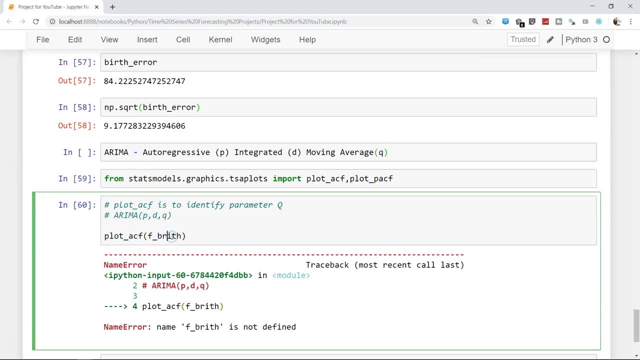 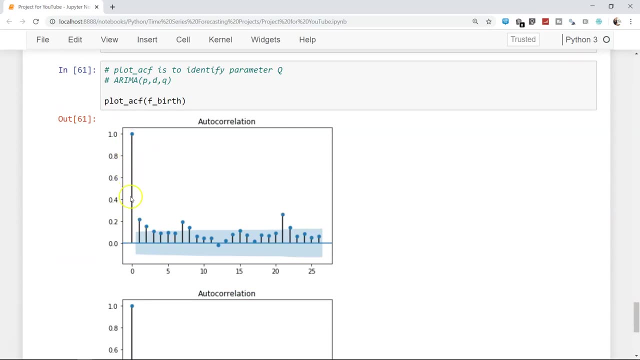 Here, but F underscore- birth, F underscore. sorry, but wrong name. And here is our autocorrelation chart. So this is the zero, That means the current value. So what it has is the correlation between the actual values and the uh. so here in this, 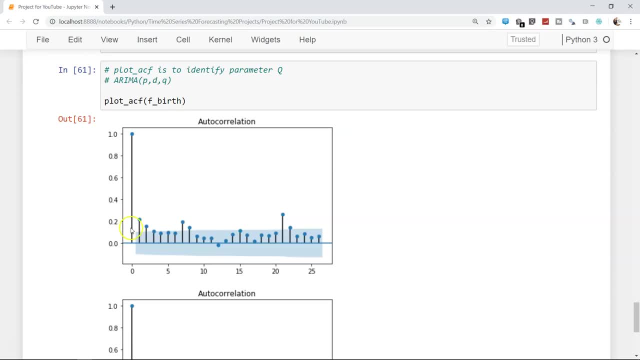 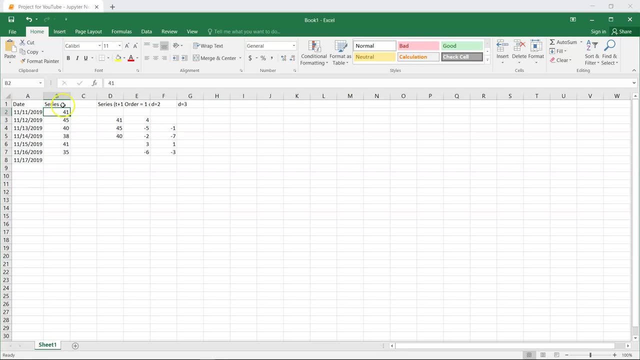 in this case. so let me go to the axle just to explain this chart. So what is happening is we are at zero. That means over here we are having the actual value as 41 and predicted value as also 41, right? 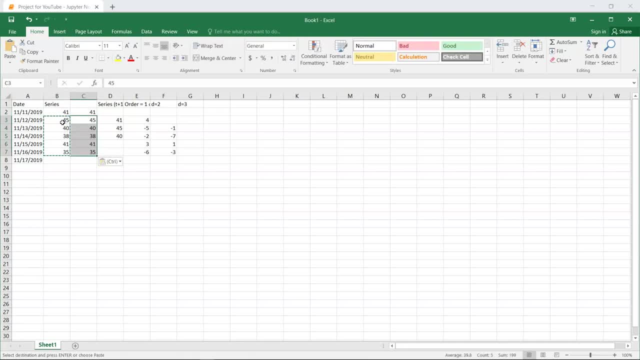 And this is so. this is what, and in this case, since you are- uh, you must be aware that correlation between 41 and 41 will be absolute. That means completely one, And that's why That's what it is happening over here, right. 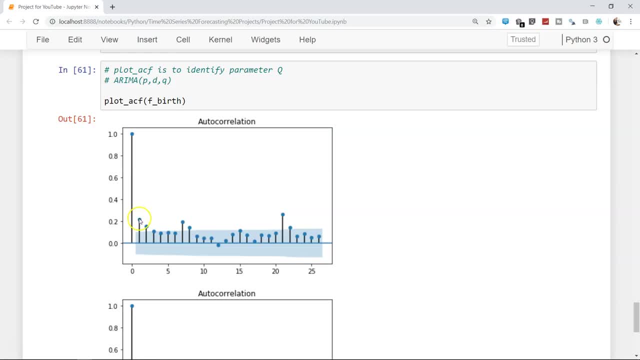 So, and when we are going to a level one, that means P equals to one- the correlation between 45 and 41 is getting checked And it says: because these are the critical limits, it clearly says that there is a correlation which is present at level one. 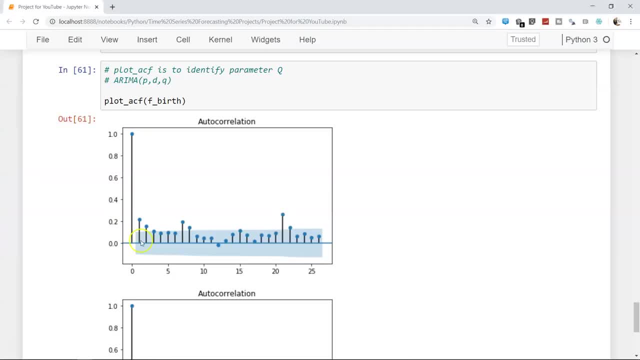 So at level two also, that means between 40 and 41, the correlation is present because it is above the critical limit. So one, two and then on third, it is under The critical limit. So what we can take is basically the first of all experiment with the P value of two. 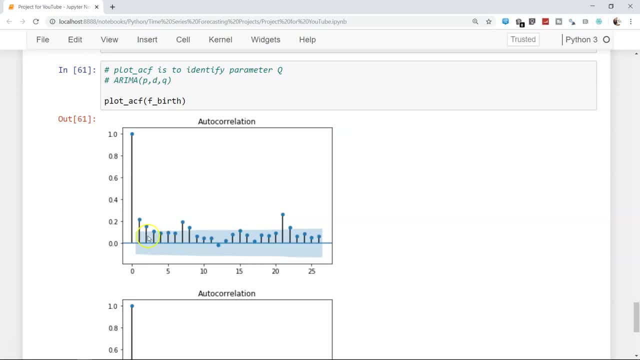 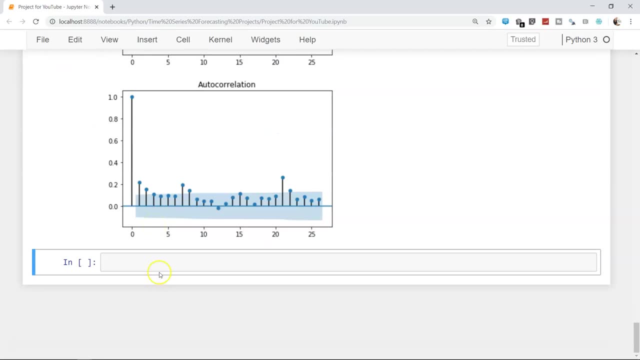 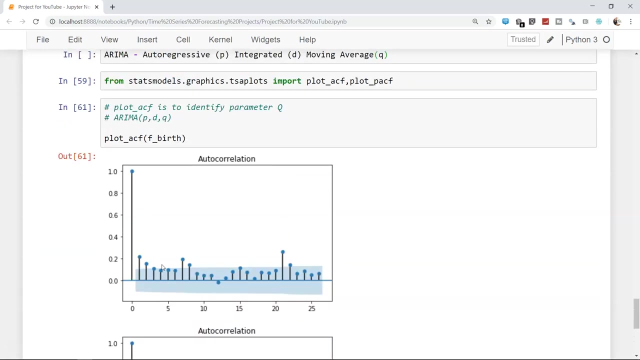 and then P value of three and maximum by four. So two, three, four is something, what we can experiment with it and then, uh, check it right. And similarly, what we have is plot underscore, P, S, C, F and F underscore, but if I'm not wrong, 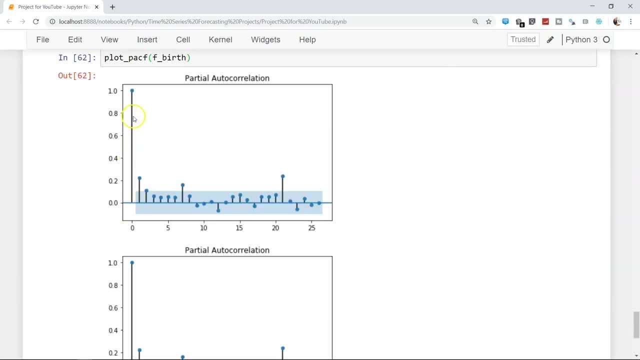 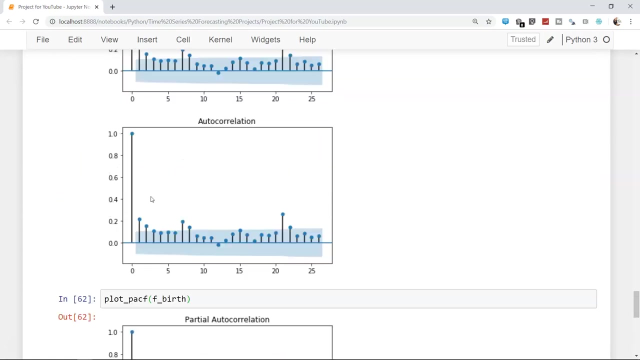 yeah, F underscore, But So after? so this is the first, this is the value, uh that we have. The first value is out of critical limits and the second value is over here, So we can check with two and three in this case. 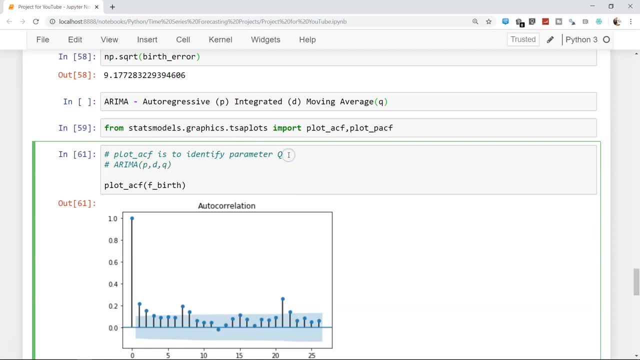 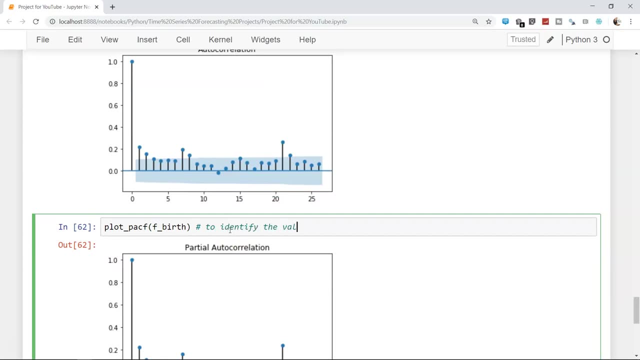 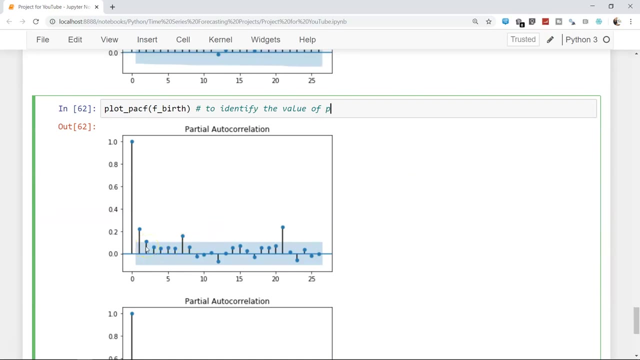 So this is plot underscore ACF to identify the value of Q and plot underscore P, S, C, F to identify the value of P. Okay, So, Okay. So let's start with uh ARIMA model, which is: uh, P is two, P and D is zero because series. 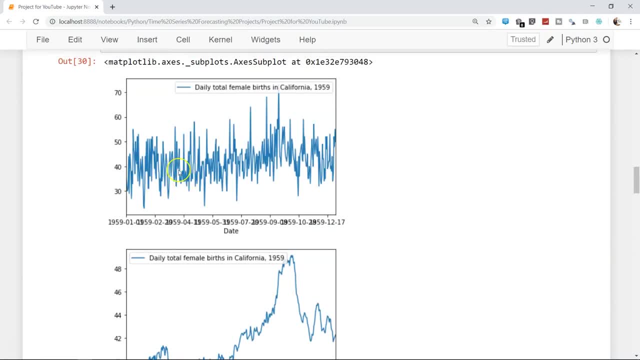 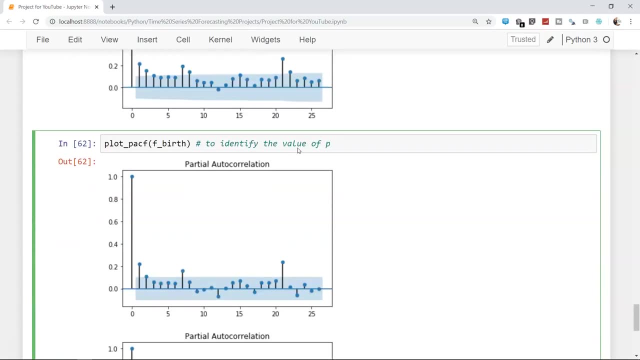 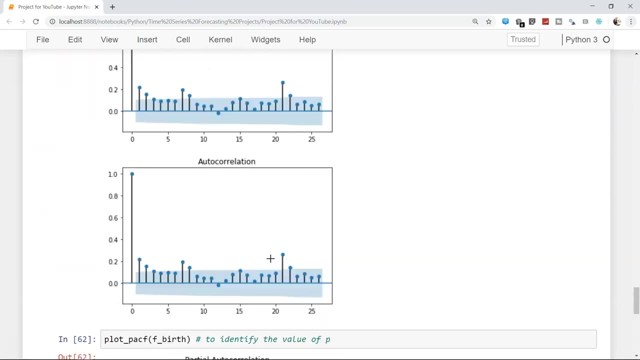 is stationary. If you see this particular, there is a very less evidence that this, this is: uh, there is a sort of a trend or seasonality that is present and, uh, we will go ahead and create a model with the help of this two, and the Q value is over here with the correlation. 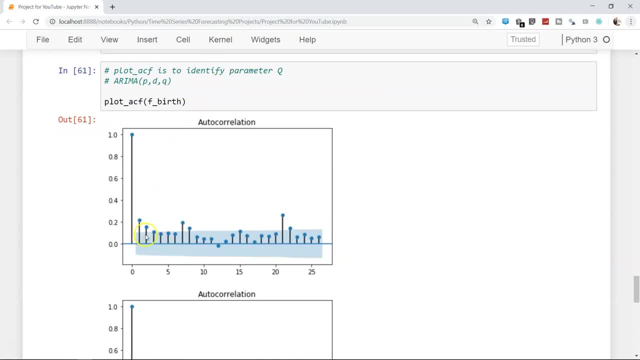 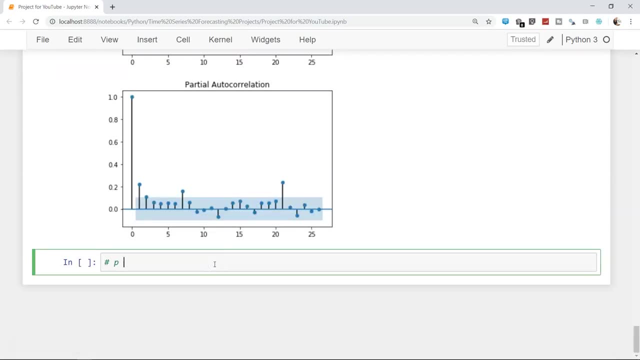 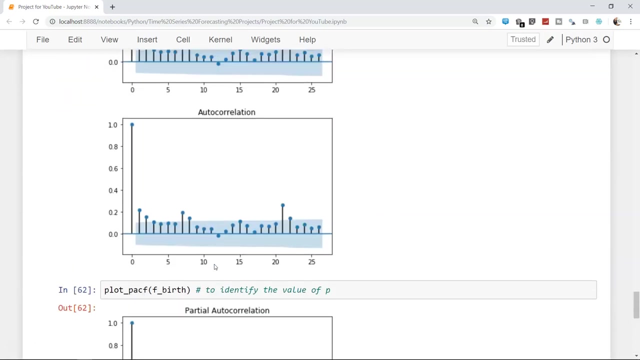 chart. So we can start with the one, two, three, we can start with two, three and four and check it. So say, P equals to two or three, and then D equals to zero and finally Q equals to two. So two, three or four. 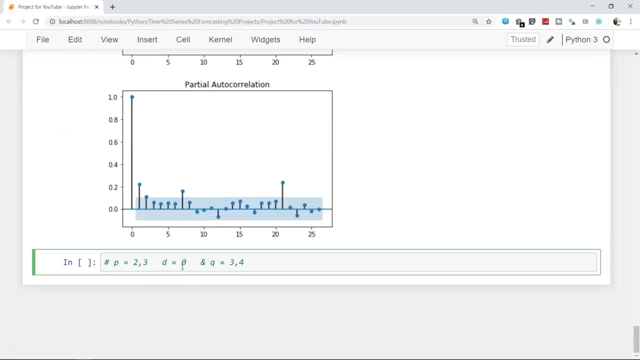 I delete two. We should not consider, So maybe three or four, Okay. So let's go ahead and create the birth before we create the model. What I would like to do is, as part of the exercise, always create the train and test. 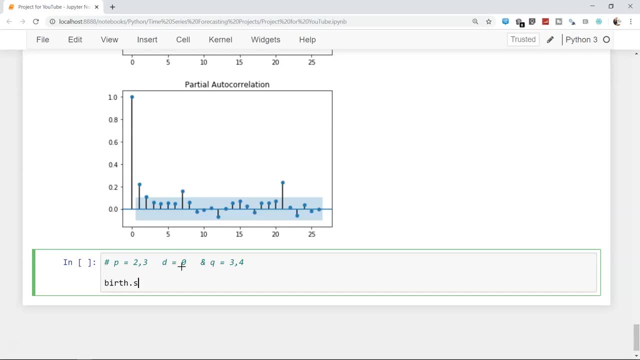 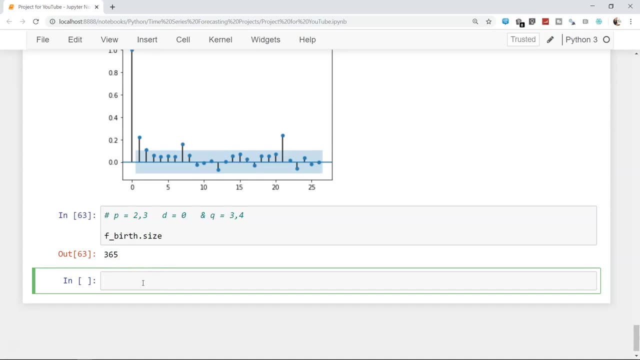 data. So birth dot F underscore birth dot size is three, 65.. So what do we do is, uh, birth underscore train, Okay, Birth underscore train, and that is zero to, let's say, three, 30 and birth underscore test. Sorry. 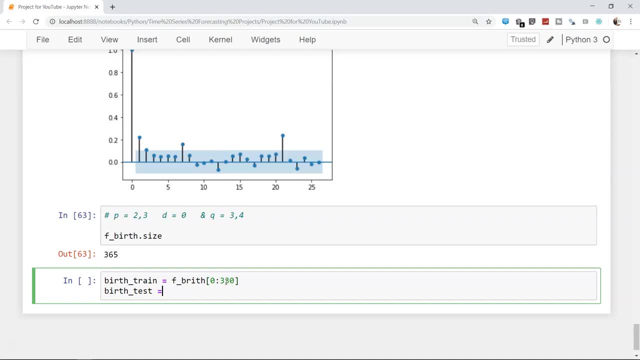 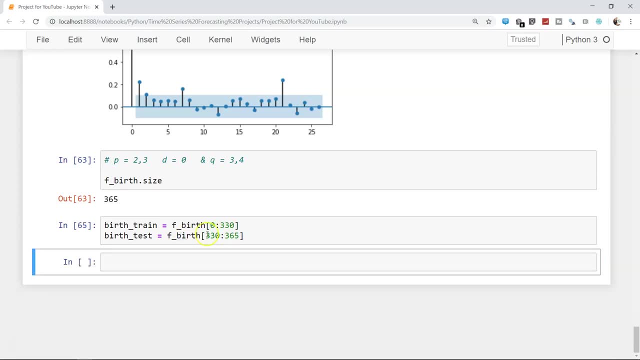 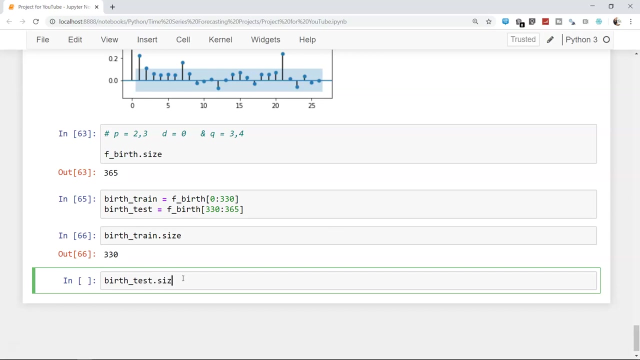 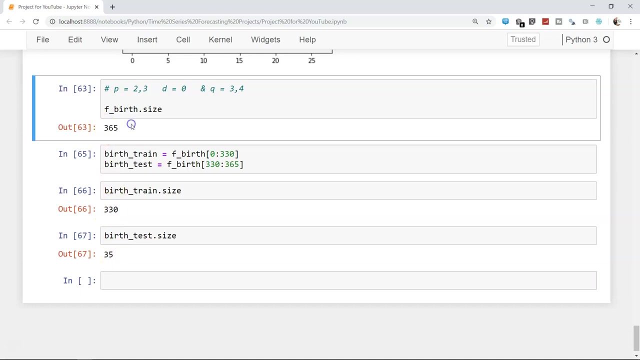 Okay, All right, Execute, Ah crap, Birth. Okay. So just to check birth underscore: train dot size: three 30,. birth underscore test dot size is 35. So three 30 and 35 is three 65. So we are covering the entire data set. 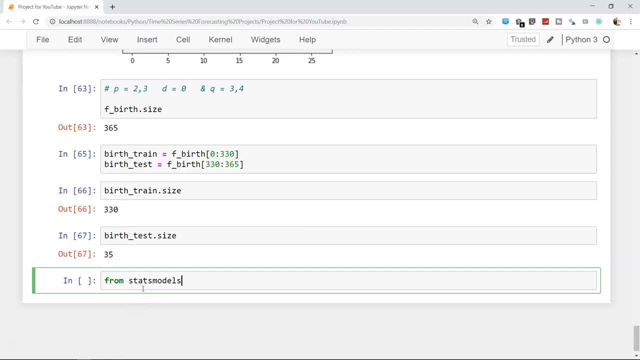 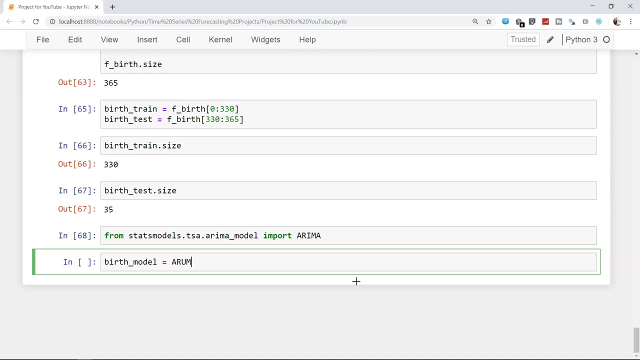 Now from statsmodelstsaar__model import. guess it should be not ar, that is only arema. sorry, the ar is autoregressive, but we want is arema. import arema, execute this and save birth__model equals to arema. 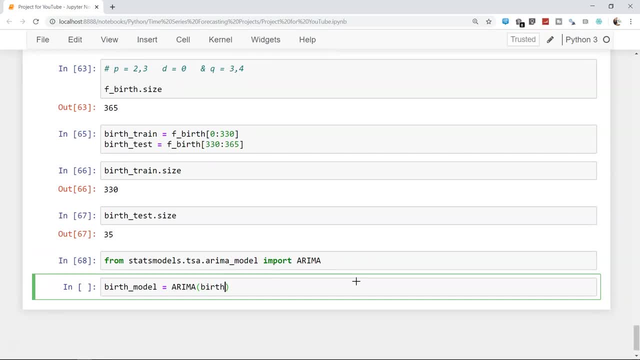 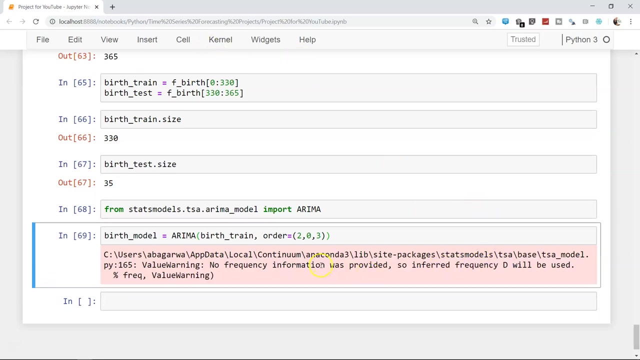 In arema we need to specify: birth__trainorder equals to, so we may say 2,0,3, ok, So In for frequency. because we have not frequency distribution, 0 is not specified. that's why it is saying: not a problem, birth__model__fit equals to birth__model. 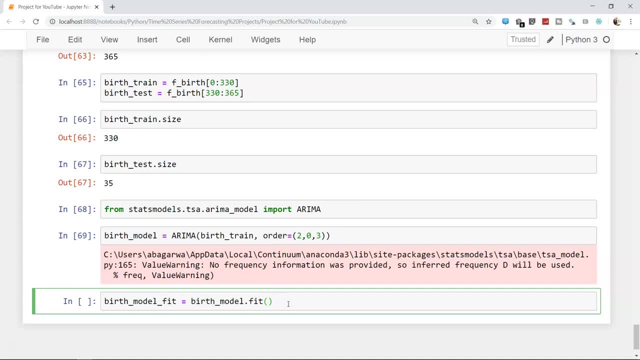 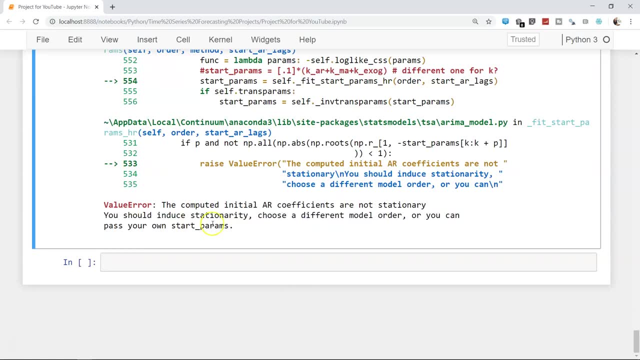 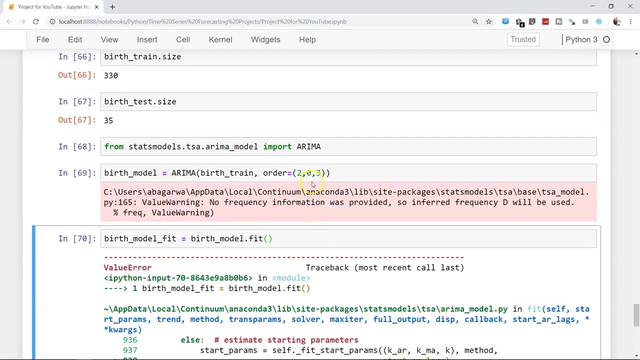 Once we fit this, we say fit, we need to fit the model. ok, there is some error. The computer initialization coefficients are not stationary. you should induce the stationary, choose a different model order, or you can pass So saying stationary. it is not stationary, so maybe we can say just one in this case. 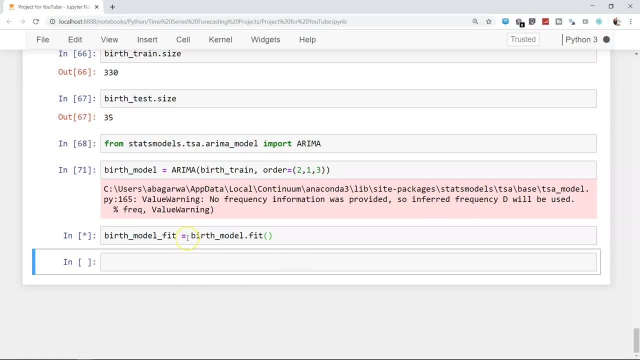 execute this, and now it is executing. So it was saying there is some sort of a trend which was present. I was thinking that from the visual that there is bit of a trend, but not very specific, but saying that we need to use the one parameter. 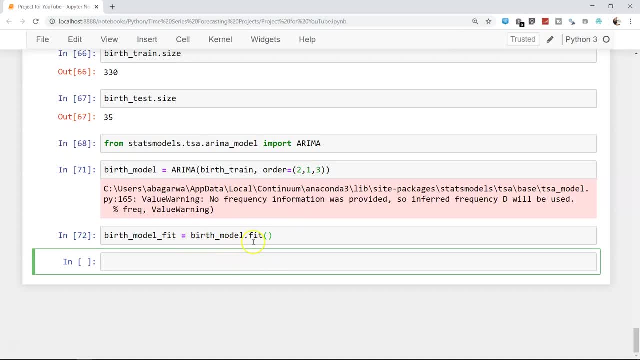 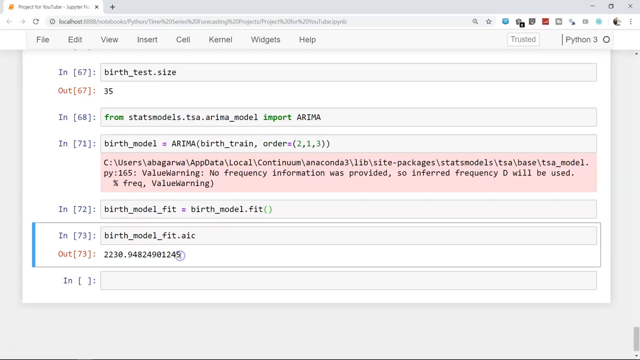 So this is something we have got so far. we have fit the model And ok, Now there is this one statistic: birth__model__fitAIC Achaic Information Criteria. so this statistics basically indicates a particular value and in general, you can read about the Achaic Information: 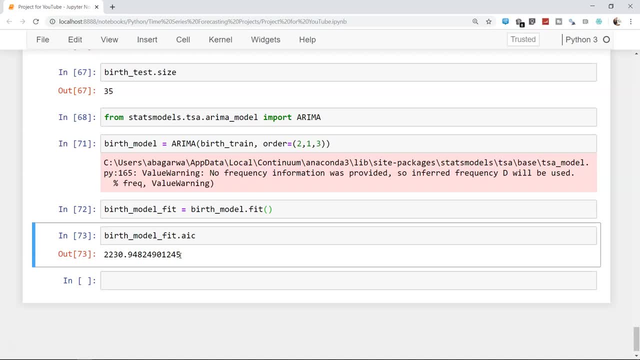 Criteria. that's a separate topic itself, but lesser the value of AIC. that means when you experiment with the order right, let's say 1,1,1,, 1,1,3,, 2,1,3,, 2,1,1,, 2,1,2, all. 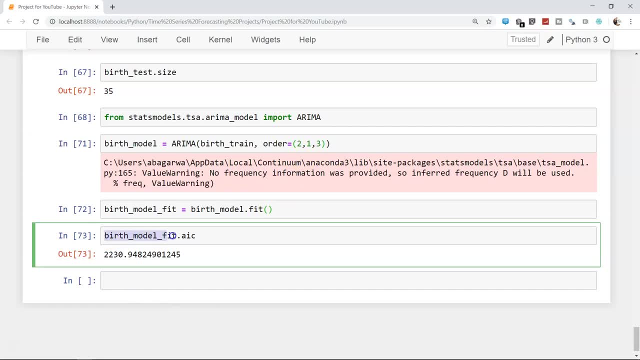 of that, you know experiment. If you do, you will see that the AIC value whenever it is less. that's the model you need to choose, basically, and that means smaller is better. Now let's go ahead and do some forecast. birth__model__fitforecast- step equals to 35.. 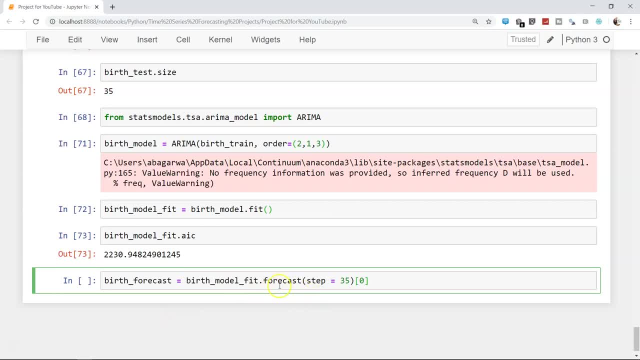 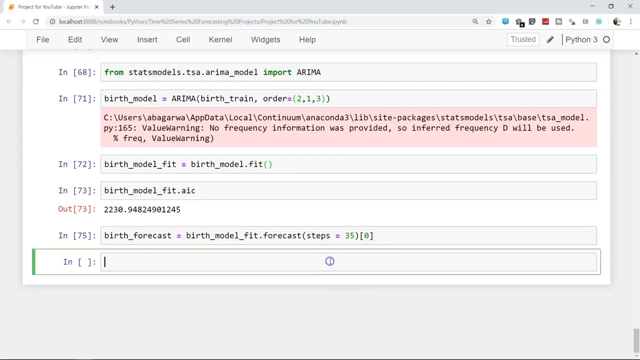 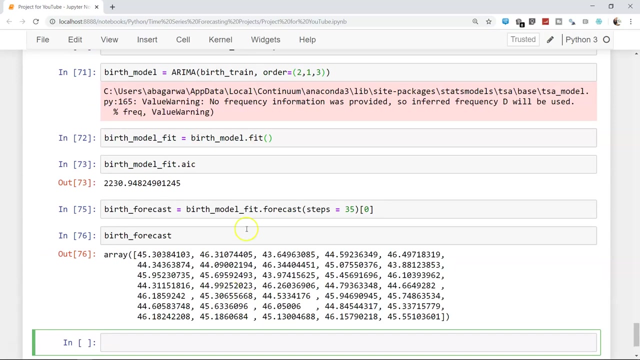 And we want the one. so it forecast gives a lot of different values, but we want just the first part of it by specifying 0, because that's what contains the forecast values. Let's go ahead and execute steps, maybe, yeah, steps, alright. so now, if I want to see birth__forecast, 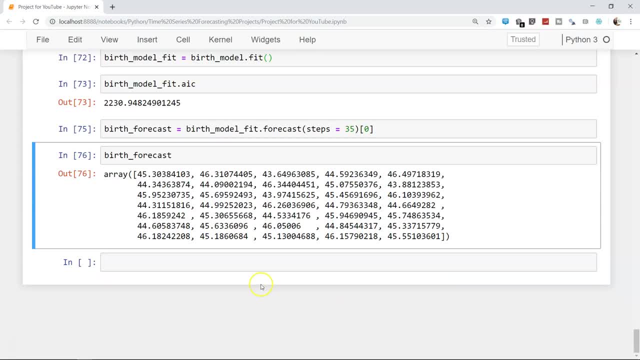 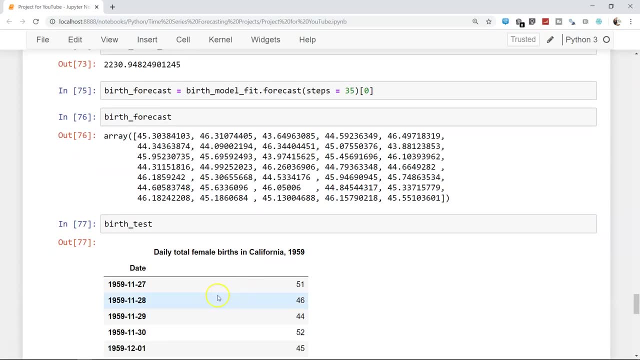 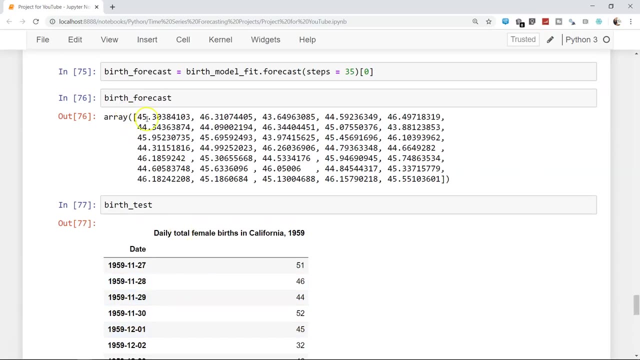 this is how your birth__forecast looks like. If I see the test value birth__test, this is how your test values basically looks like. These will be your 35 values. So what we forecast is 45, but actually we had 51.. 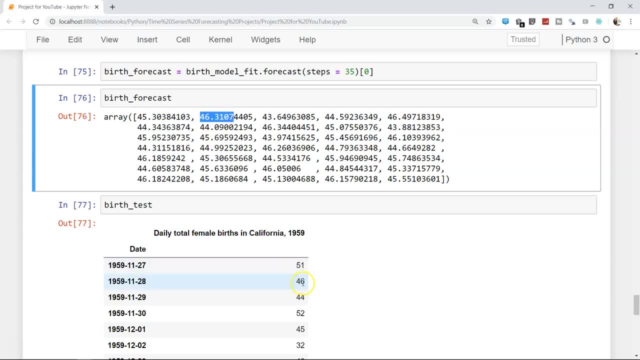 What we forecast is 46, and actual value is 46,. that means very close. What we forecast is 43,. actual value is 44,- again, very close. What we forecast is 44. But the actual value is 44.. 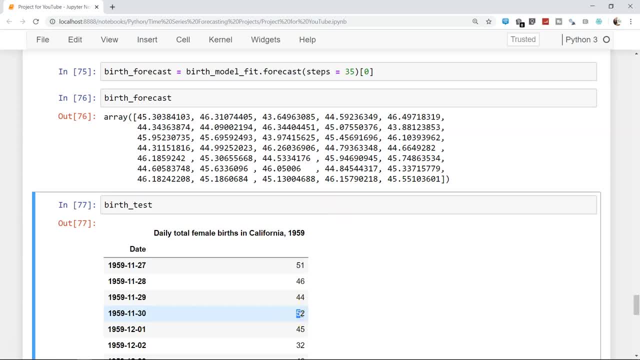 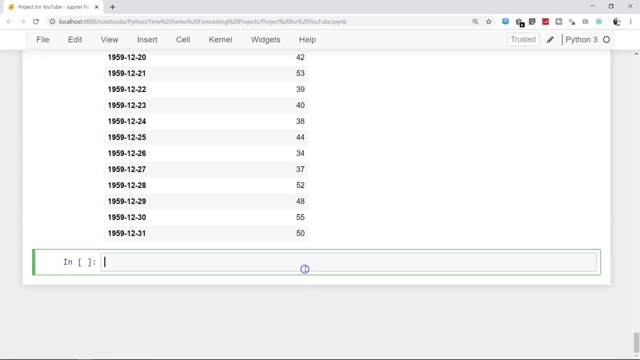 The actual value is 52.. So you can see that in some cases we are predicting really well, in some cases we are not predicting that good, And that is part of this. is just normal. I mean, that happens when you produce the. 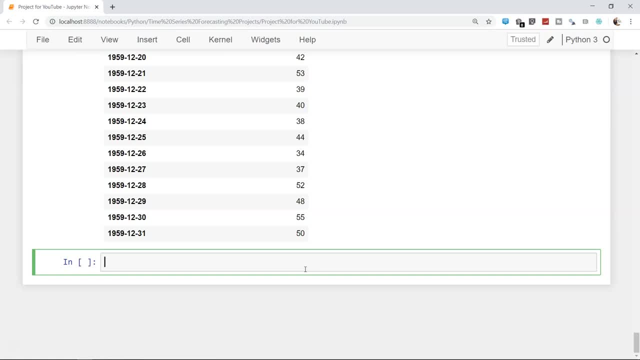 model. nothing is perfect, otherwise there is no point in doing all the experimenting. But with experiment you can always reduce the error. So now let's go ahead and try to see the error. So same method: npsqrt mean squared error. 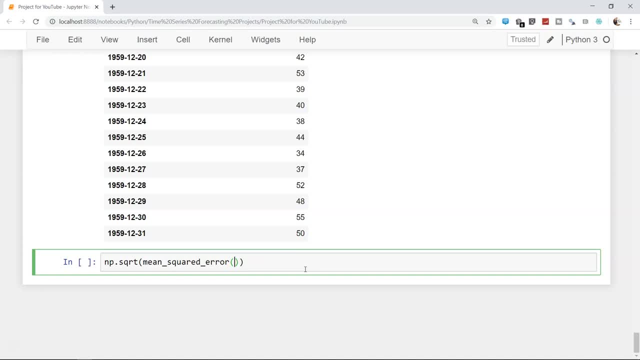 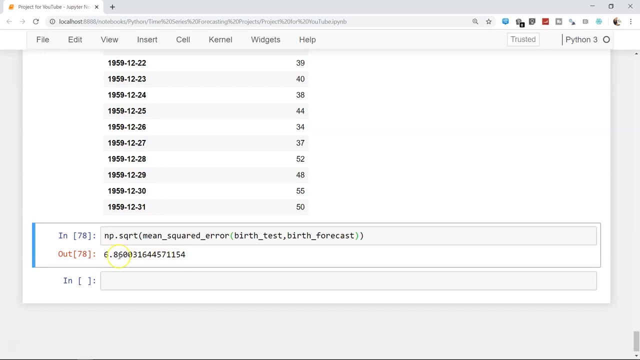 And within that, I think first is the actual value. that means birth__test and then birth__forecast. Let's compute this. The value we got is 6.86, and it is better than our model. what we created is the naive. 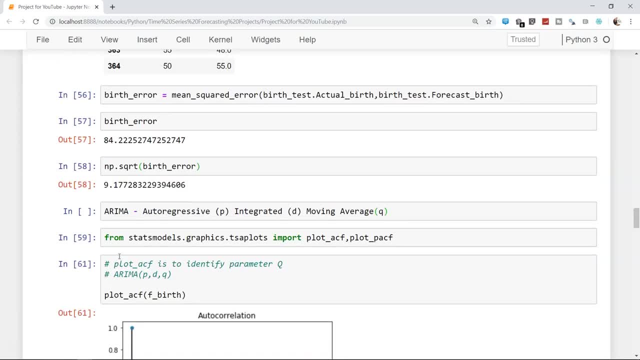 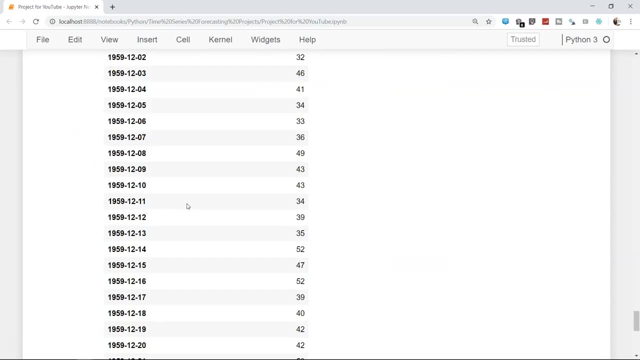 model over here. So if I go up, yeah, this is here 9 point. There was an error of 9.16.. 9.177.. But then we got the error of 6.86,. birth every day. 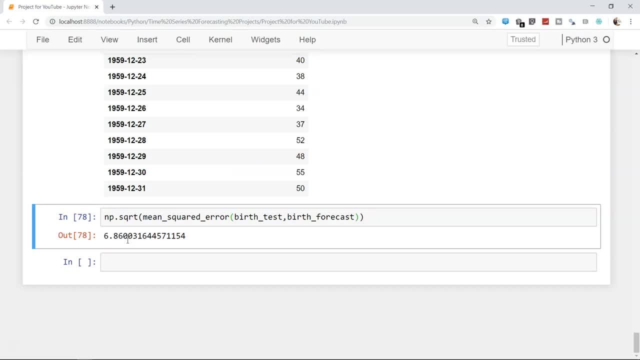 So we reduced to 3 births, And that means we are doing a better job in this case. Now there are many things which can be done to further improve it. Either you can be satisfied with this, because this is again a very low score. I mean very. 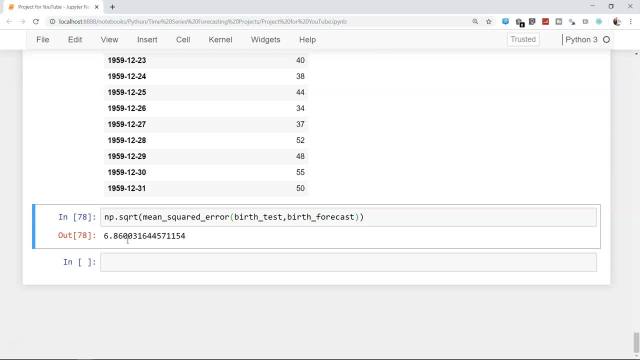 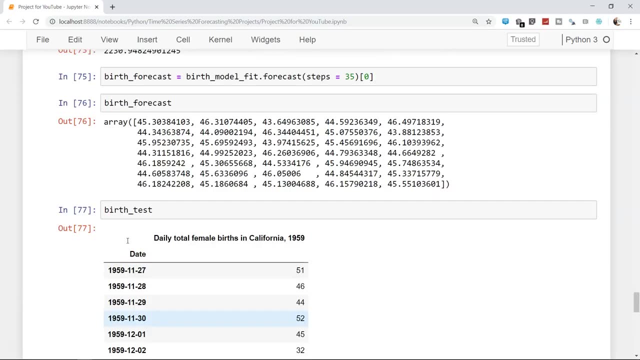 good score. the low is better in this case because we are very near to what. how much birth, How much birth is happening every day in California. But you can further improve it And how you improve. it is basically going to here, say 213.. 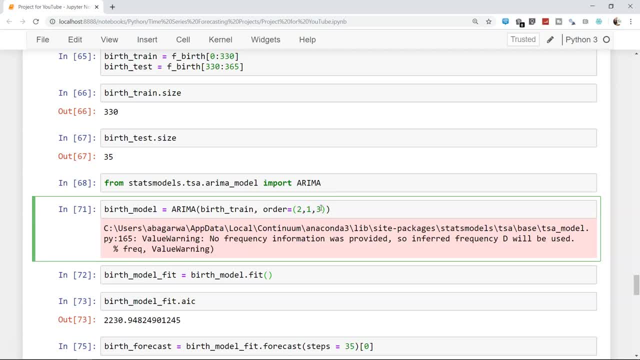 You may say 111,, like I said, 211, 213, or maybe 211, 212, all the different orders that you can specify. There is a way by which you can automate the entire order, but for now I am not specifying. 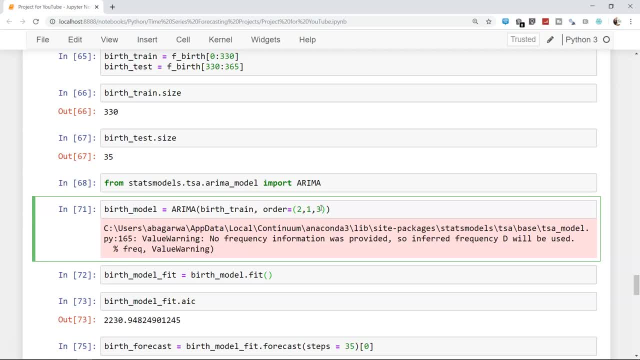 this. I really want you to experiment one by one so that the more you will repeat, the better you will become in doing all of this operation. And after that, once you specify, I would really like to see your comment that what you have done. 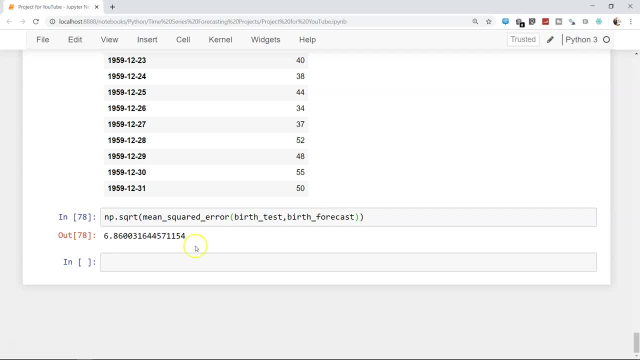 And you can take it up as a challenge that how you can reduce this value to something which is 4.. So that's a improvement of almost 3 points, because right now we have six point eight, which is almost seven. but if we can reduce to something four or four point five, that would be really great. 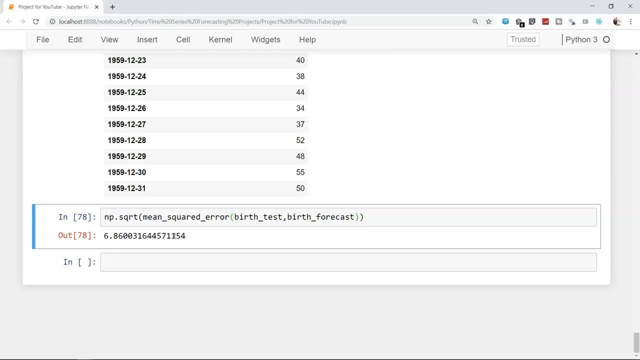 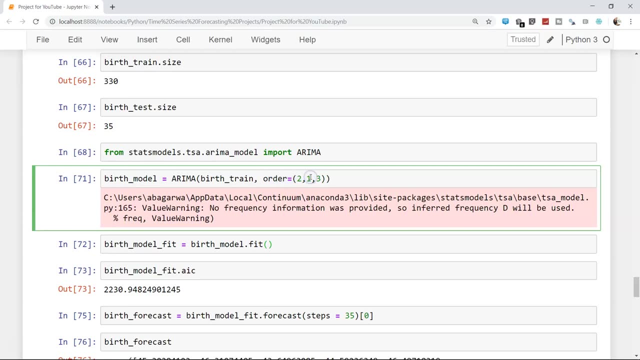 and I would really love to see what you have done to improve it. other way of improving it, apart from what you have it over here: the specifying the order. other way of improving it by normalizing the data or standardizing the data or doing the data transformation. there are a couple of techniques which are there for 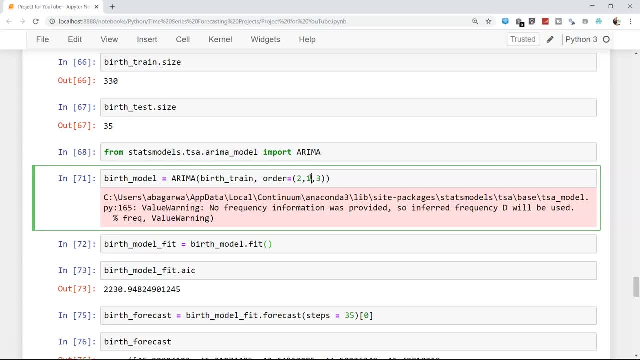 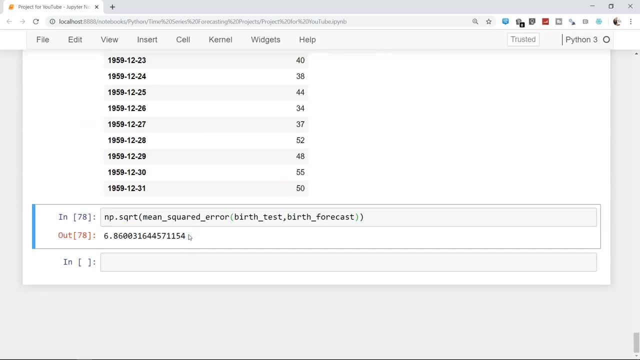 data transformation and I will share it with you in the next videos. but those techniques really help you to bring it, bring the value down. so there may be a scenario that it may bring down, but there may be a scenario it may not bring it down. but it's all part of experiment, as part of the data science. you are a 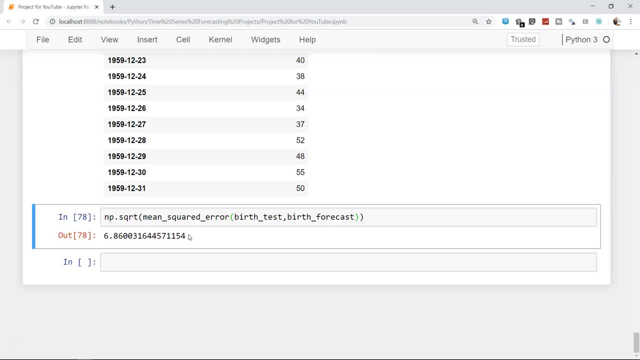 data scientist and the data scientist, the scientist- whether it's a data scientist or any other scientist, the scientists job is to keep doing the experiment. it doesn't really matter that you are getting very good result or very bad result. it may happen to it that you may get the worst result and you feel like 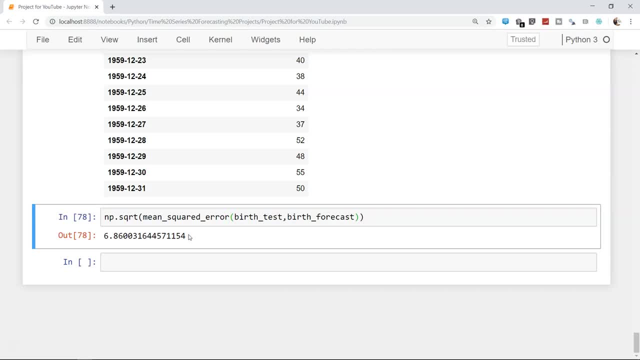 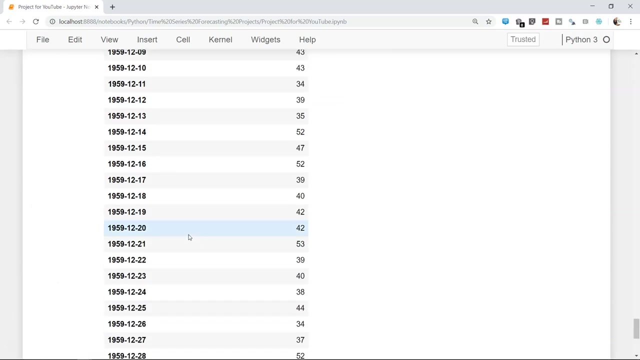 oh, why did I do it? but that's not the case. you have to keep on experimenting. the more you experiment, the more you learn about it, and you will actually become the real data scientist, but not the one who just run the algorithm and it's done. so I would really like you to to test all of these different techniques.